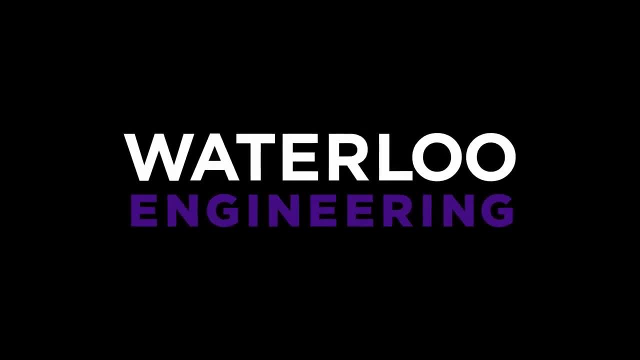 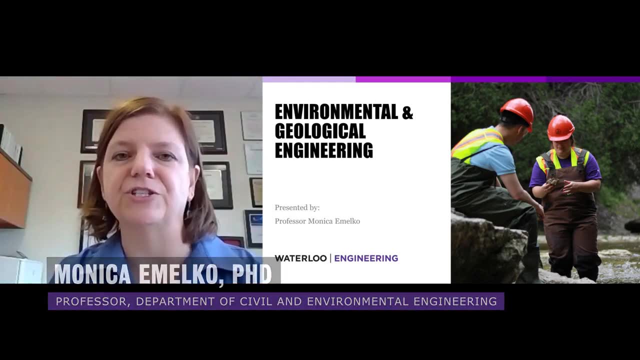 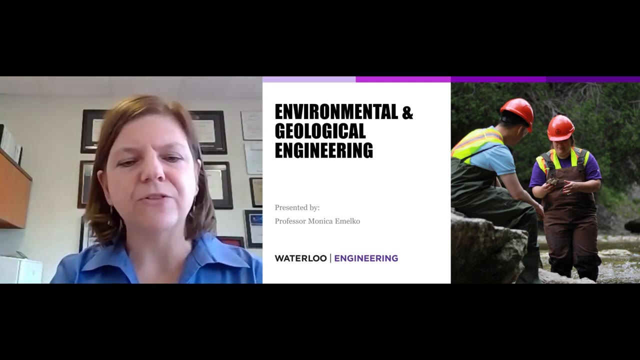 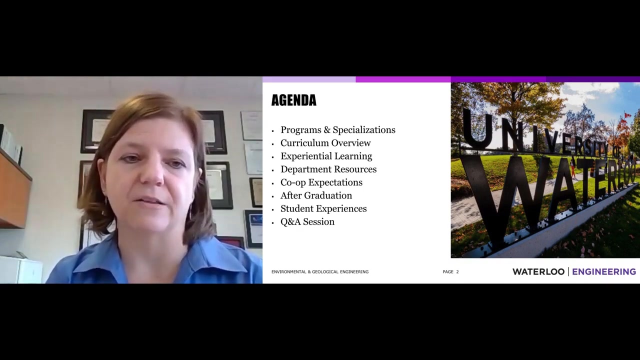 So let me tell you a little bit more about our programs, Environmental Engineering and Geological Engineering. They're both housed in the Department of Civil and Environmental Engineering at the University of Waterloo. I think you'll be surprised, they're not what most people think they are. So what I'd like to talk with you about today is our programs, what we have both in the classroom and outside of the classroom, because it's much more than just classroom study. We've got a co-op program, we have all sorts of fantastic departmental resources and we're really interested in getting people to where they want to be after graduation. And again, that's a lot more places than you might be thinking of when you hear the words Environmental Engineering and Geological Engineering. Then I want to tell you a little bit more about some of our student experiences and then ultimately tell you how to get in touch 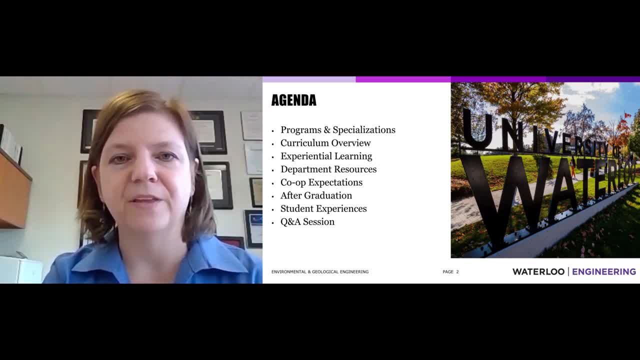 with us if you have any questions or you just want to learn more about what we're doing. 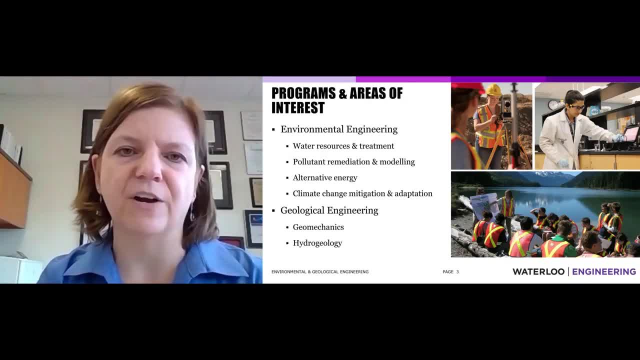 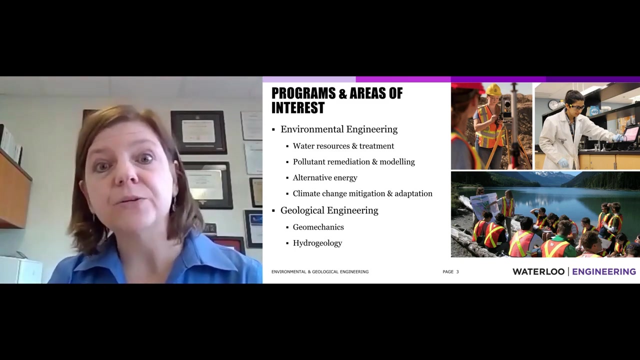 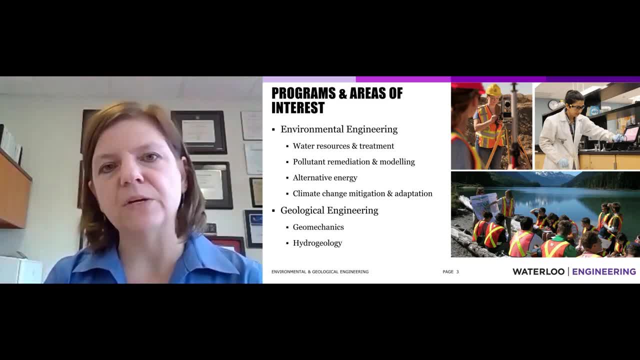 Is it safe to build on? Is it safe to breathe? What do we need to do with it to make sure that people can interact with the natural environment to the best extent possible for their comfort and their safety? And of course, as you can imagine, climate change, both mitigation of those impacts and adaptation are massive issues that we necessarily have to undertake. 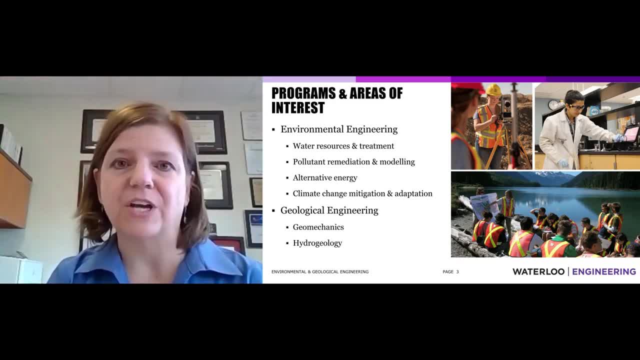 engineers necessarily lead those discussions. And so when you think about engineering, every aspect of engineering needs an environmental engineer. And when it comes to the environment that we interact with, geological engineers are there to help guide us in assessing risks and how we interact with land that we build on and preserve, and also how we interact with resources 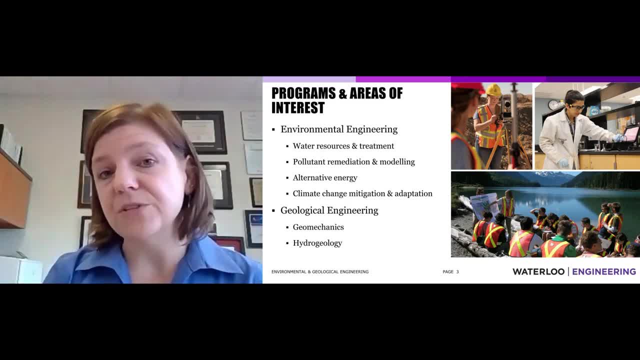 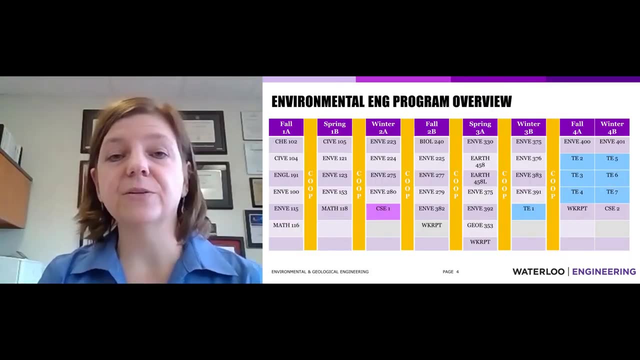 that are found on that landscape. So for example, subsurface water supplies, and do we have enough? How do we interact with it? Can we preserve it and make sure that it's safe for all water values ranging from ecosystem diversity to drinking water? So let's talk a little bit about the 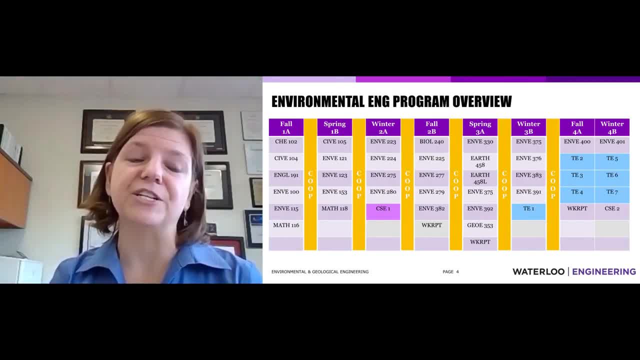 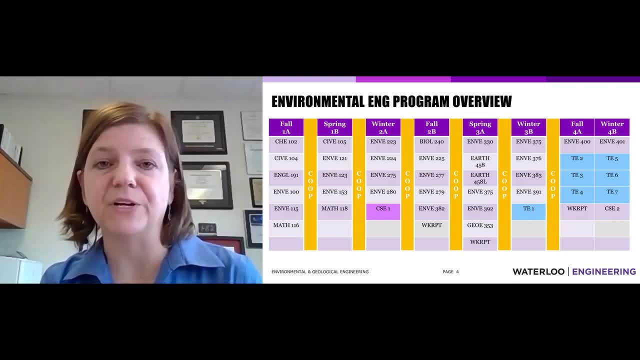 programs that you'll be having inside the classroom as environmental engineers. So you should see here right off the bat, we have a term of coursework, and then we go into a term of practical experience in our co-op program. And that pretty much alternates throughout until we get into fourth year. You can see that we've got a lot of requirements. We've got a lot of requirements 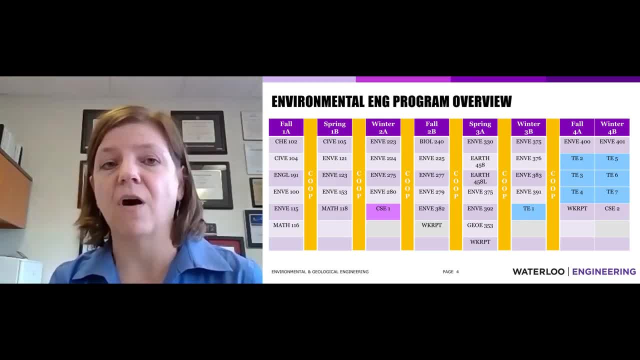 that require technical courses, but also a wide range of complementary studies electives and tech electives that allow you to choose the paths that you want to specialize in, both with respect to your interests and also to the technical areas that you might want to specialize in. One of the things I'd like to point out with respect to our program is that you come for the fall term, and then immediately in January, you're already getting valuable working experience and getting paid for it. And we've done that on purpose. That's something that allows our environmental and actually our geological engineers as well, as you'll see in a minute, get out into the workspace in January, get that valuable experience and not be competing for jobs in the summertime when most university students are out looking for jobs. And so we see back in the classroom, and it's actually fun to be in the classroom in the summertime, because summer courses tend to be a little bit more relaxed. And that works really well with making sure that people get the most they can out of their educational experience. 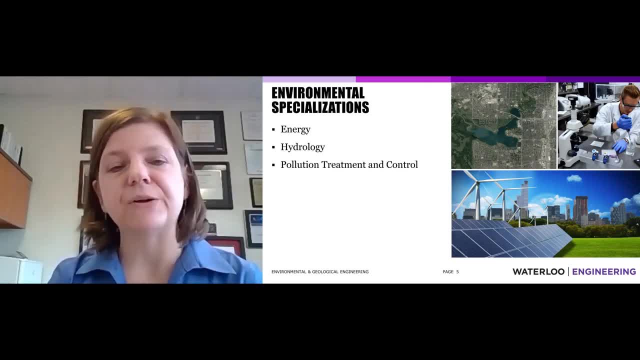 So when, it comes to then those programs, I mentioned that there are different options for specializing with 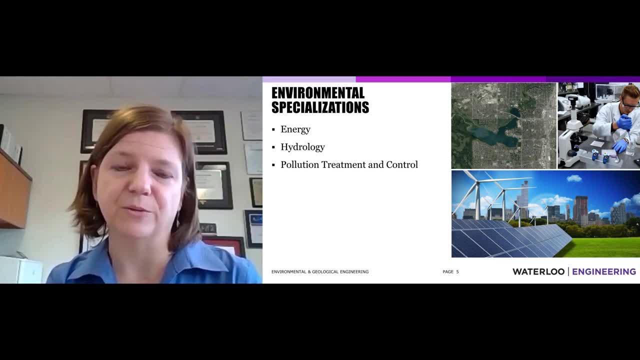 respect to both your technical program and then moving beyond your technical program. So in the environmental engineering program, we have areas that you can focus on and we call those specializations. So as you can see here, they have a broad range. It can be energy, alternative energy sources, efficiency with energy, can be green energy. It can be water supply, and that's what hydrology is. Hydrology is the study of water. We also have individuals here at the university who look at pollution treatment and control, and we're referring to that as pollution here because it can be water pollution, air pollution, and soil pollution. 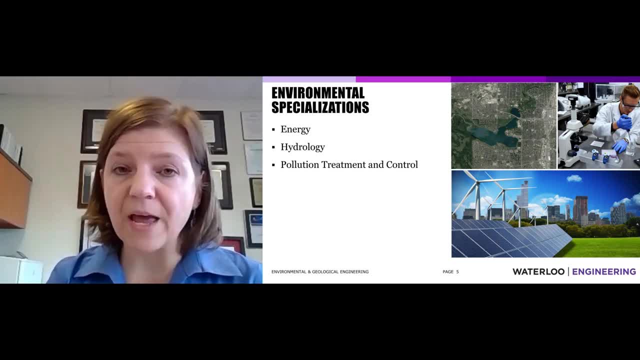 So we're looking at aspects of both when that pollution occurs, how do we clean it up? But also, again, when people interact with society, What can they do to make those interactions more positive, more environmentally friendly? 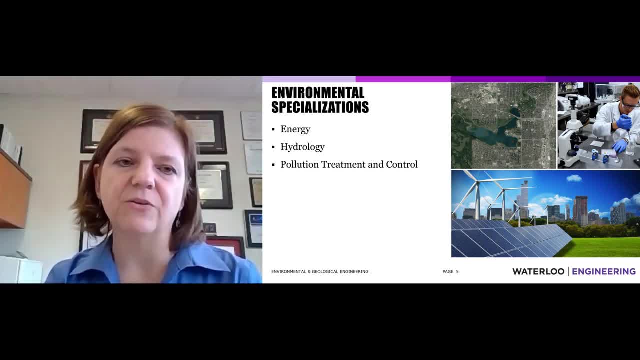 You need environmental engineers to engage with the whole community, but you also need to bring in those process leaders, and to create a network of people that manage that. You need to bring in those process leaders, and to create a network of people that manage that. you need to bring in those process leaders, and to create a network of people that manage that. engage in those discussions because they're the ones that specialize in understanding those interactions and what we can do to not only mitigate but keep interacting with our environment 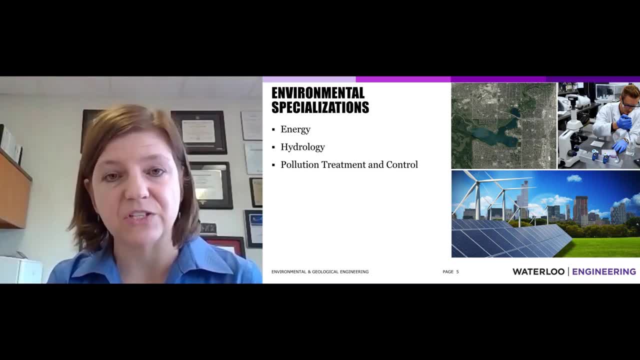 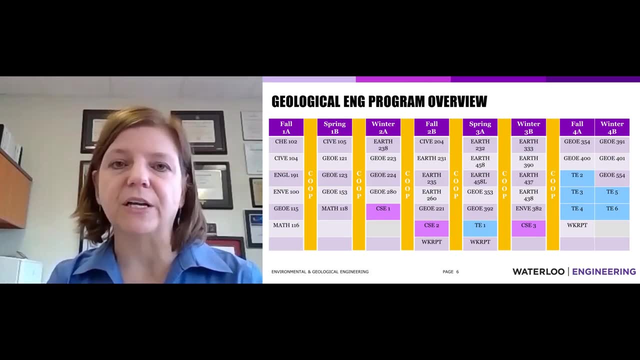 in a very sustainable way that means we'll have access to those resources not only now but in the future as well. Our geological engineering program is very similar to the environmental engineering 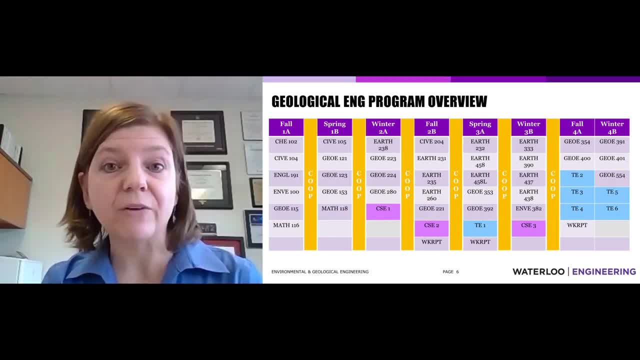 program with respect to its progression. So like the enviro program you see that we have alternating terms starting off with a school term in the fall and then going on into co-op in the the winter term and then coming back to school for the spring term. So again you're not 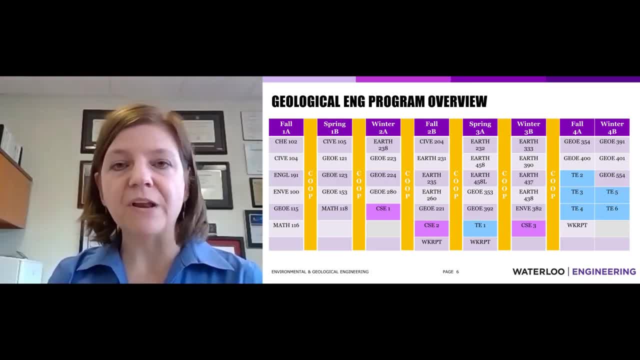 competing for jobs when there's peak demand and then what that actually allows you to do is when you go out for your second co-op term you're going to be that much more competitive because you're 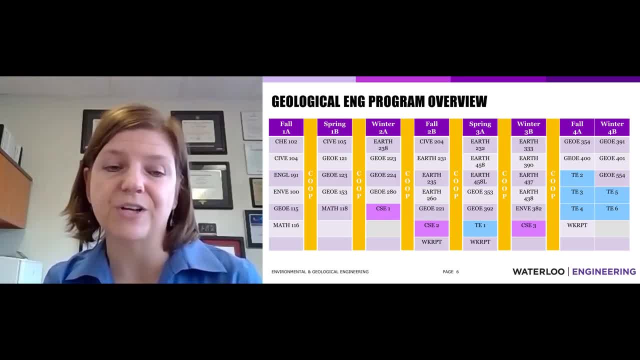 going to be getting those jobs in your first co-op term that are highly sought after. You can see 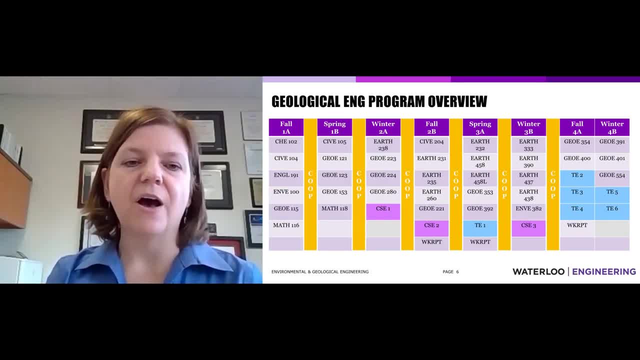 here again we have the same progression between electives that are both complementary studies so things like policy things like economics but then also technical electives that it might allow you to specialize in whatever area of interest you have that goes a little bit deeper than the overview of what is a geological engineer what is an environmental engineer and 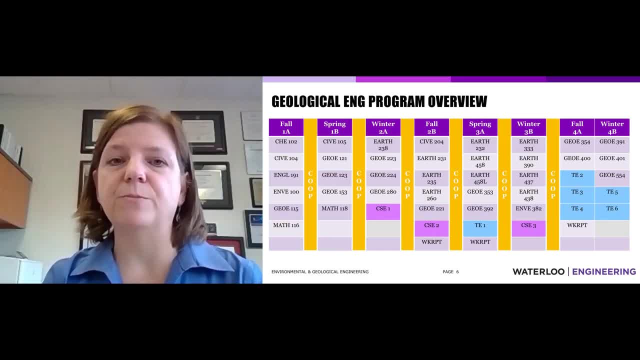 you can see that progression here. I should point out that for both programs fourth year the terms are back to back and one of the highlights of that is having a year long or at least in this case it's two-thirds of a year long because it's two terms 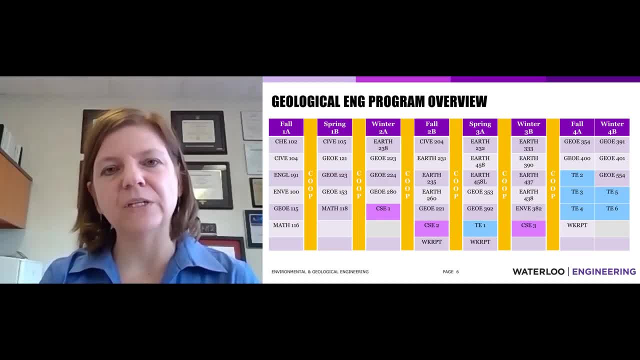 a design project that spans across those terms that really highlights capacity and interest of our students. I'm going to talk about that in a little bit so hang tight we'll talk about that some more. 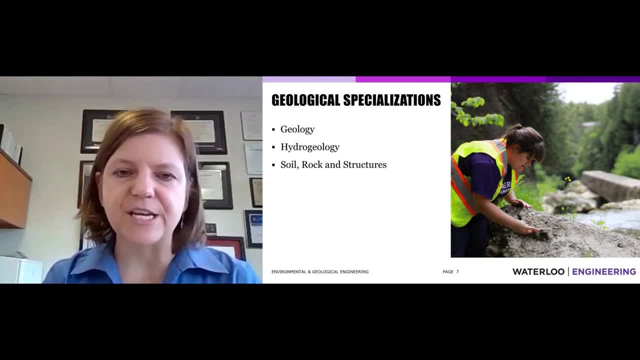 In the geological program we also have several specializations and so they can range from geology what are the materials that make up the landscape that we live on. So if you think about Canada for example we have a unique geology that even though we say we're very similar to our neighbors to the south in the U.S. our geology actually means that we have different risks relative to our neighbors and they have to do with our history of glaciation. So our surficial materials are different when we're building when we're thinking about water supplies when we're thinking about hydrogeology so that's their the amount and quality of water in the subsurface and our structures in general are natural infrastructure structures. So our soils are rocks. 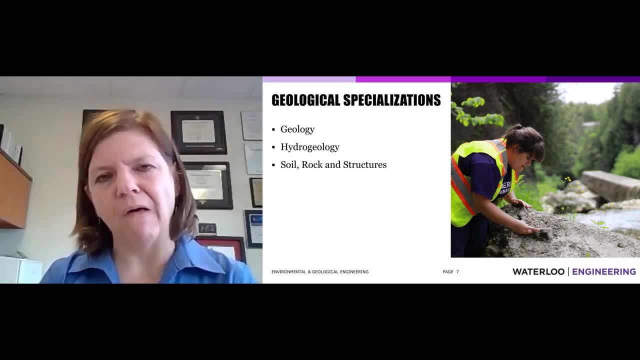 How and how we can put built aspects of the environment on that landscape we need to think about is it safe are there going to be risks and are those risks going to be exacerbated with naturally occurring disturbances that are exacerbated by climate change so these include fires floods. So we need to think about how we interact with that environment and sustainably survive in that environment and with our communities and with our interests in including of course. 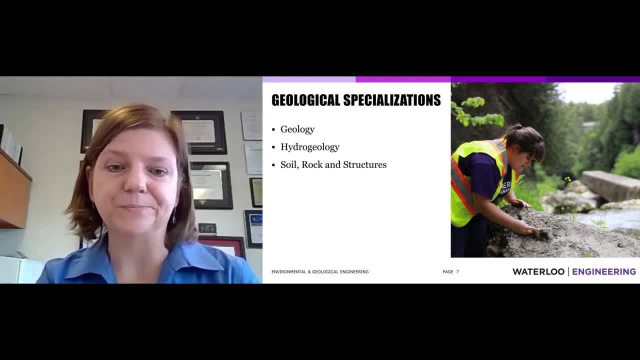 Being able to. Sustainably live on this planet. 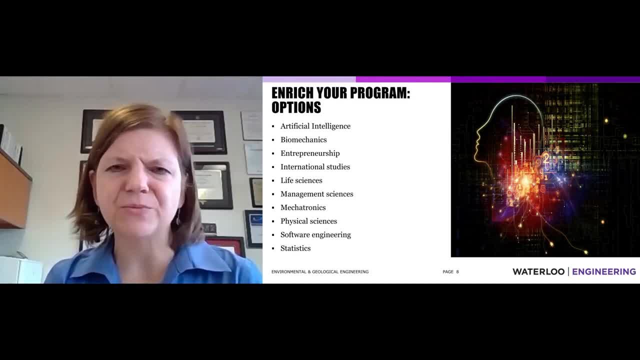 Now we can further enrich our programs because of course we don't work in a vacuum. In environmental engineering and geological engineering we necessarily are the department and the programs of I like math and science. Our science disciplines are tools in our understanding and math is the language with which we make decisions about science. 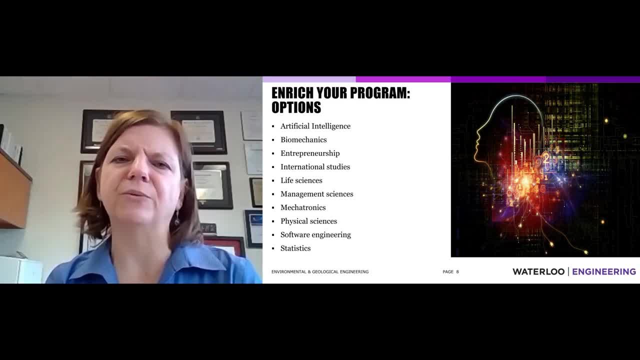 So we have opportunities to strengthen or enrich our experiences in the undergraduate program. So we have opportunities to strengthen or enrich our experiences in the undergraduate program. 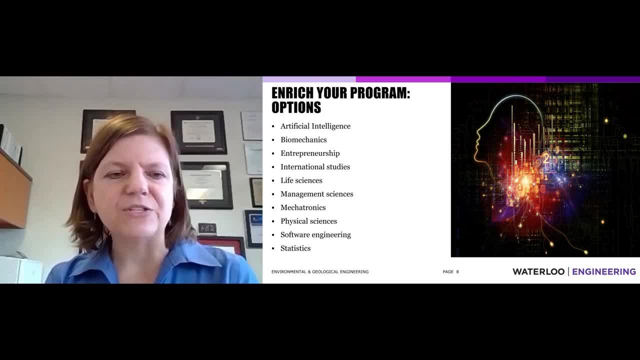 Use those skills andülme. 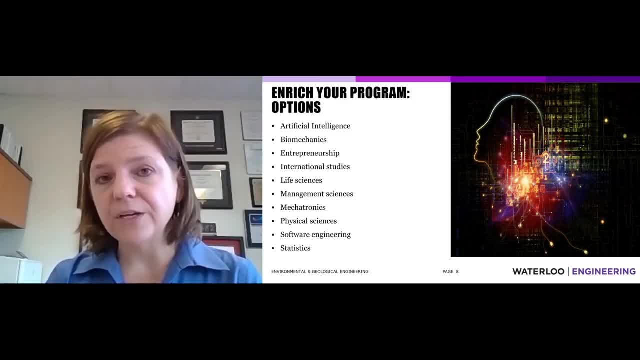 So these are the four elements, we definitely need through the curriculum depending on what areas of math and science you're interested in. So we've got some of those listed here for you. Certainly one of the ones that is on the forefront of many peoples minds is artificial Intelligence. We are now going into an age where. Where machine learning and data streaming and analytics are at a new level, we need to think how do we as engineers, as applied scientist in, It makes you that our society that we live in really feel at home to make sure that our organization that we live in, our institutions that we live in, really feel at home to develop. Make sure that the society that we live in really feel at home to implement. We're gonna need to think about. 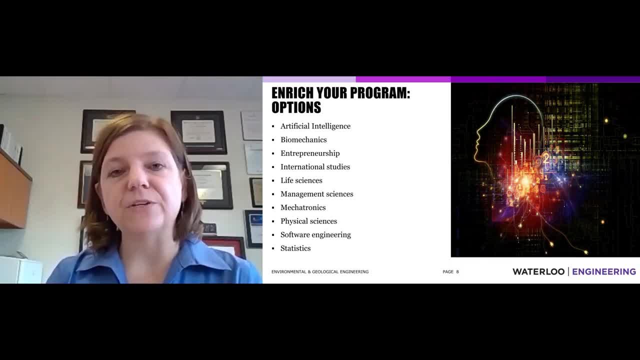 We are here today, we know most inhabitants are displacement of these new génillos and the best we we due to live this beautiful Chinese and American. 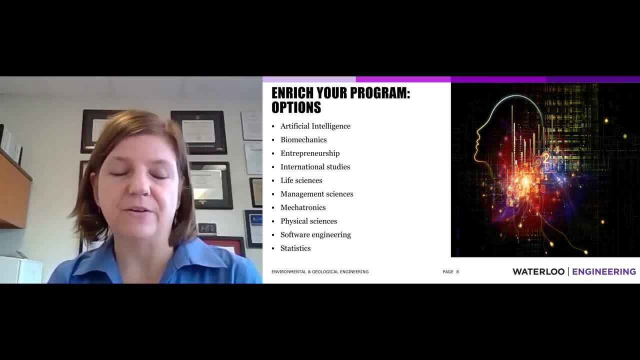 comfortable with these technology driven solutions that they feel that they can count on the decisions that are being made not just by people but by computers it's going to be an interesting time and as engineers we take neither a dystopian or nor a utopian attitude about that but rather a science driven perspective and so really we are going to be the leaders of the future helping decide society decide how we make decisions so this is an extremely exciting time to come into civil and environmental engineering department and work in either environmental or geological engineering programs but it's not just limited to computers and math we need to have subject matter expertise as well because those programs are only as good as the information that goes into them so you might be interested in management philosophies and strategies or you might be interested in the life sciences and connections to health you might be interested in how do we put together the software that's going to make these 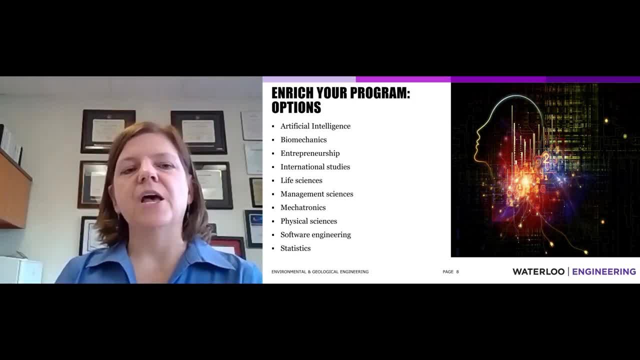 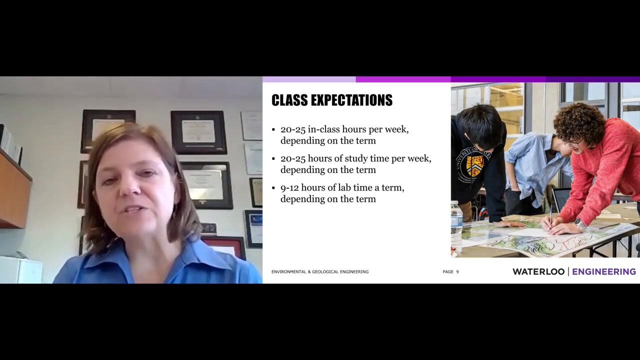 decisions how do we quantify these decisions and risks so you might be interested in statistics for example all of these options are here at the University of Waterloo with world-class experts that you can connect with so that you can be making decisions and making them based on the best available science and math approaches to those decisions and so this is engineering it's an involving field and it necessarily means we have to be able to work with others from other disciplines now in terms of our classes this is this is an area where you might be a little bit surprised yes the University of Waterloo is a very large University and our Faculty of Engineering is world-class and it's very large however that doesn't mean that students become numbers here so we have a very targeted and focused strategy with respect to what we expect from students and how we want to interact with them so in the classroom as you might expect there's typically a good number of hours of classes in the classroom classroom expectations typically range from about 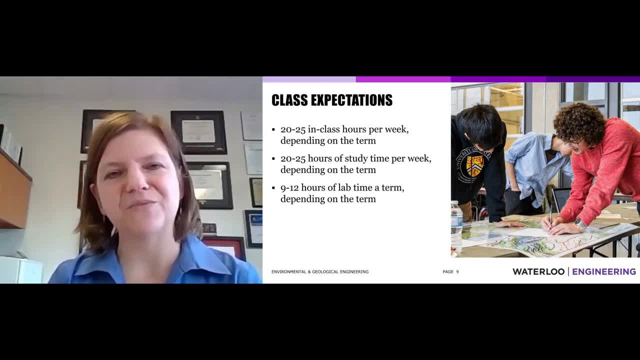 20 to 25 hours per week depending on the term in the specific classes you're taking of course but the difference between high school and university is a straightforward one there's in-room class in classroom learning and there's also outside of the classroom learning one of our goals is that you will become lifelong learners how do we go about that well there's a whole lot of enrichment that occurs outside of the classroom and that might be in the form of lab time it might be in the form of non-structured time you'll find at the University of Waterloo there are a lot of study groups and various opportunities to work in that non-structured time and I'm going to talk about that in a minute but I just want to summarize that overall as an undergraduate student who's a full-time student you're pretty much working a full-time job and that job is 40 to 50 hours a week so there's the classroom time there's an equal amount of outside of the classroom time and really that's true for most university we do have a good deal of hands-on time 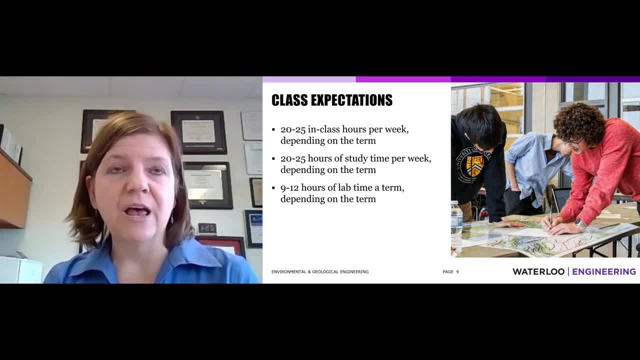 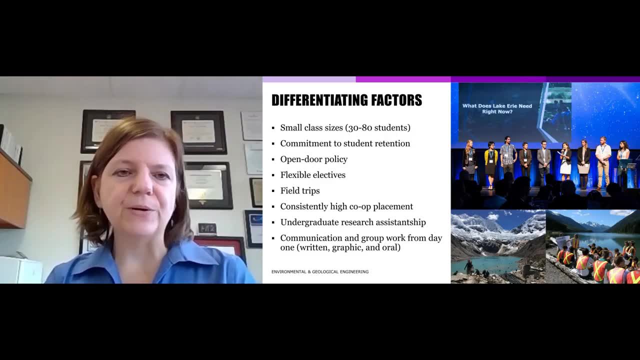 in labs whether they be design labs or science labs and then also we have other formats for evaluation and so I want to talk a little bit about those so in our programs now specifically so this is in environmental engineering and geological engineering I think you'll be surprised to find that you're really not a number I always think about how amazing it is that I remember students from 15 and 20 years ago and a big part of that is our philosophy of education we necessarily keep our classes small let me tell you tell you if you get into our program it's because we want you and you belong here. We have small class sizes they're very competitive anywhere from 30 to 80 students between the environmental and geological engineering programs. As demand increases because it's one of the fastest growing sectors in engineering for jobs we might increase those programs in size a little bit but we certainly won't increase them a lot and part of the reason for that is is we have a commitment to open door policy approaches. We want to interact with the students and get to know them and make sure that they're advancing not only in their academic career but also in their personal aspirations for their professional development more broadly. So connecting with various aspects 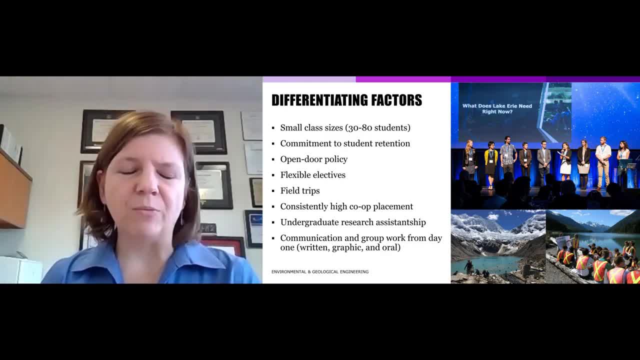 of industry for example. So consistent with that open door policy is trying to advance your whole 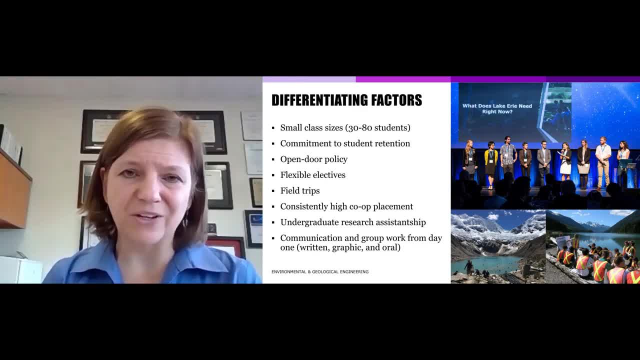 growth as a student and as a professional not just whatever might be occurring in any one class and so that means getting to know you. 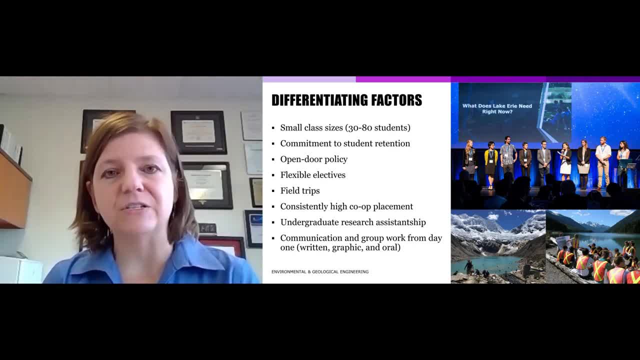 And being able to live up to our retention to once you get in here we want you to stay here. We want to help you in whatever it takes recognizing that it's a big transition from being in high school to being in university. We just talked about how it's a different style of learning but there are also other challenges that you face and it has to do with learning how to interview for jobs, being able to provide you with feedback on your resume, being able to help you advance your interests. So we have all sorts of opportunities to help you with that. 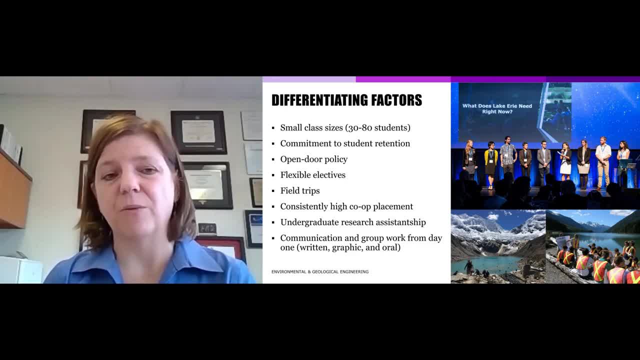 The supports in place where we can interact with people but it starts with an open door policy. 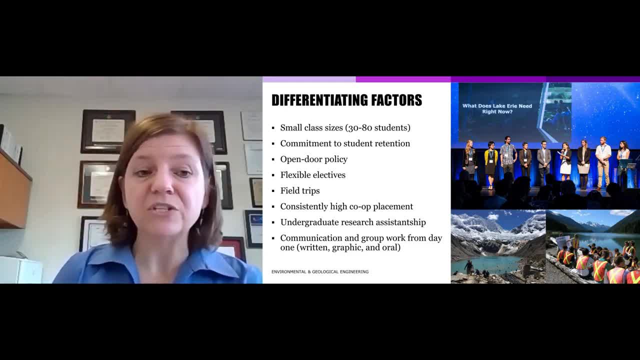 We have opportunities to explore research undergraduate research opportunities, the URA program. We have opportunities to support you in your co-op 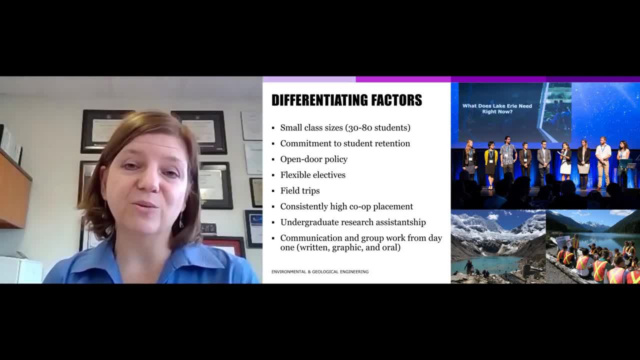 placements. So connecting with employers both while you're looking for employment and when you're not. And you'll hear about that some more but we have wonderfully high placements almost entire placements every class. And of course then there's the professional development. 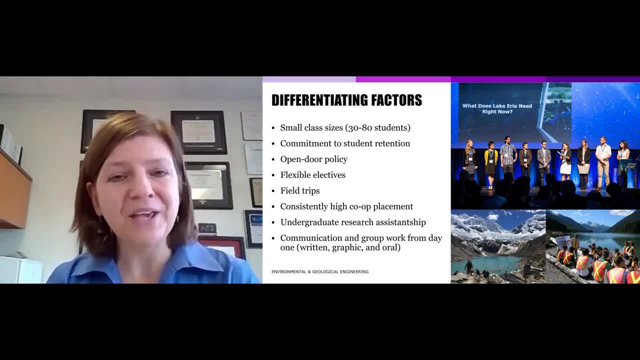 doesn't matter how brilliant you are if you can't communicate that brilliance then that's not going to get you very far with respect to development in your career and also with respect to development and impacting the world you live in and the world around you so communication is a huge part of what we do communicating your ideas communicating that brilliance communicating the ideas of groups 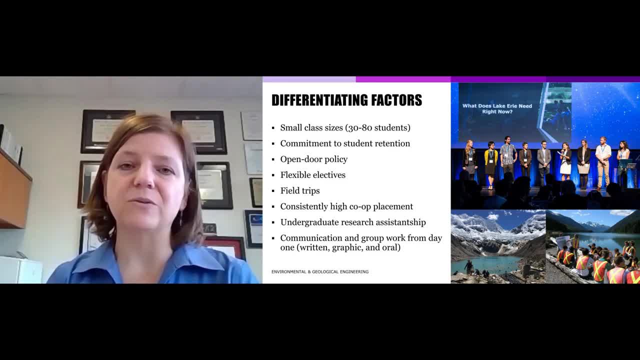 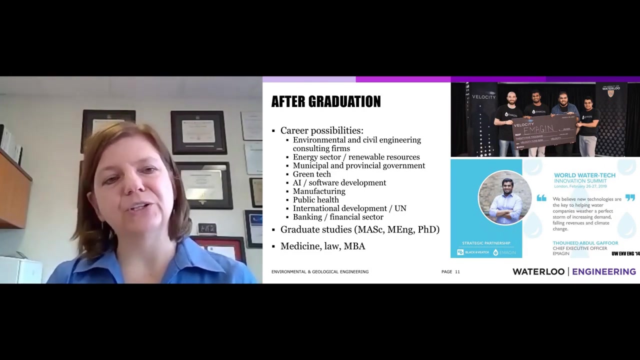 because multiple heads are better than one with respect to solving the big problems of today the wicked challenges that we are faced with the wicked problems of things like climate change adaptation so how can we maximize the impact of the science and math that we are learning that's what it comes down to and that doesn't stop while you're an undergraduate it also then transcends into how you interact in the future it's a it's quite incredible how many of our graduates come 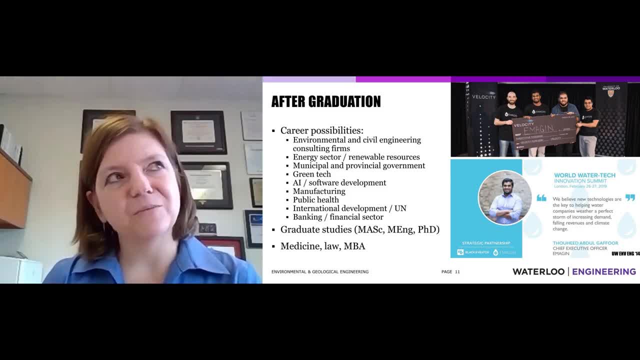 back and interact with our students and part of that is is because we're all we're all professionals just at different points in time in our careers after graduation there's a range of jobs our students work in and you might be surprised to find that they're not limited just to engineering because of the diversity of skills that we develop and topics that we touch upon our students coming out of the environmental engineering program and the geological engineering program can really take on any number of challenges and the way I describe it I think of it as engineering gives you a critical thinking set of skills and that allows you to take on any careers that you might imagine so yes a lot of our students go on and work in engineering whether it be consulting green tech the energy sector public health even the banking and financial sectors and international development but you'd also be surprised to find that a lot of our students go into medicine law business programs and that's because our programs give you a good solid basis and critical thinking and communication of that critical thinking and then what are you ultimately going to do with that it's going to be to solve problems so engineering is actually an outstanding basis for pretty much any of these problem solving oriented professions it's a great 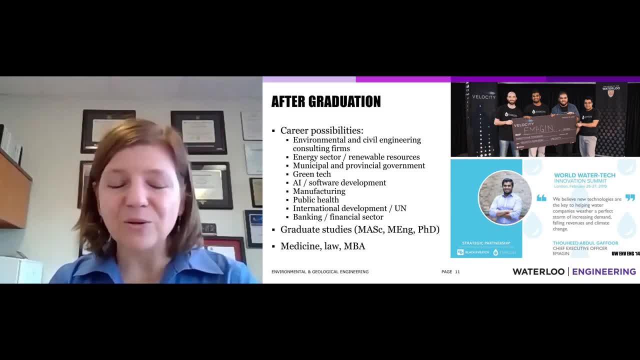 way to go and yes some people stay in engineering a lot of people go into graduate studies but a lot of people go into other professional programs I have a neat slide here which I think shows exactly that this is a slide that I'm going to show you and I'm going to show you a slide that I'm going to 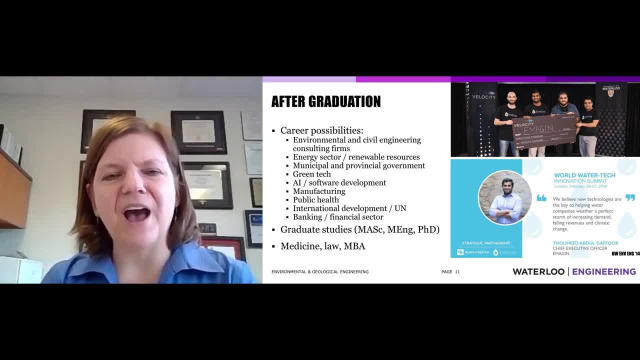 slide outlining one of our competitions that we had for design projects and I think you've probably 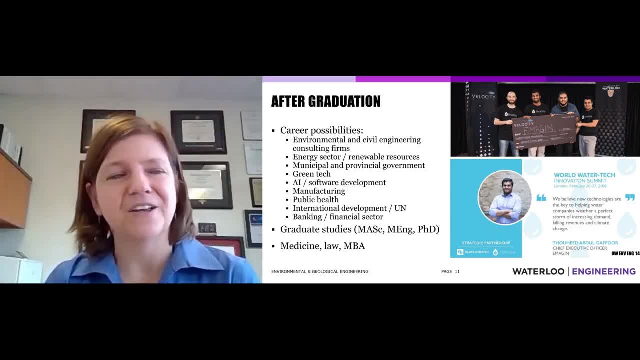 heard that at the University of Waterloo there are a lot of startup companies because why not if you can have an idea you can identify a problem build a solution there's a lot of need and interest in in getting those solutions out to impact society that's what we're all about this is one of our 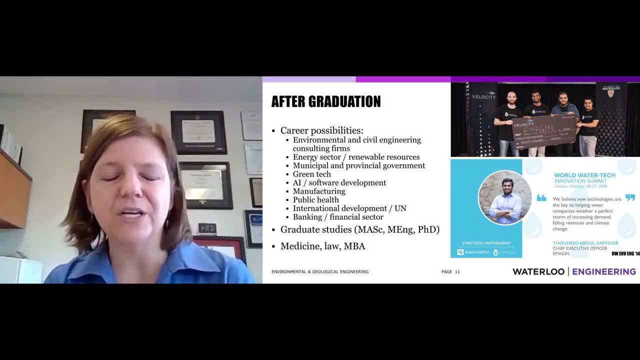 undergraduate students who graduated in 2014 Tauheed Ghafoor so he graduated in 2014 stayed on for a master's degree in engineering and he's a graduate of the University of Waterloo and he's a 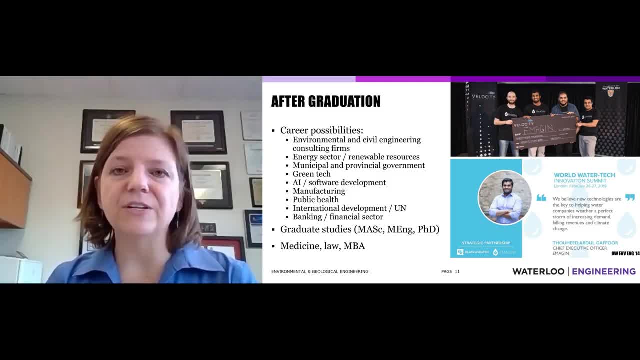 graduate of the environmental engineering program and this year in January the startup firm that he and colleagues from Waterloo started up it was called Imagine and it's all about bringing artificial intelligence into the drinking water sector they're literally one of the lead companies if not the lead company globally with respect to bringing AI approaches to the sector of 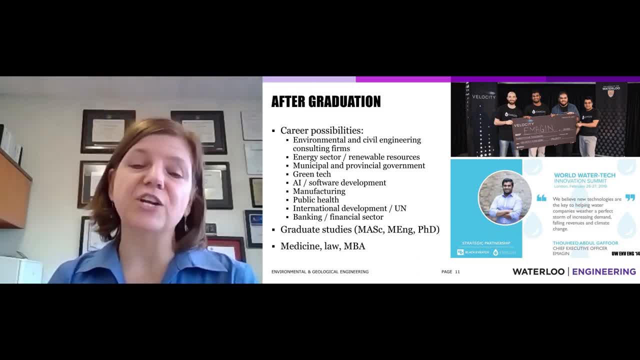 water supply and water treatment globally this January they were bought out by Innovise so they're no longer Imagine they're Imagine as part of Innovise Innovise is a company that 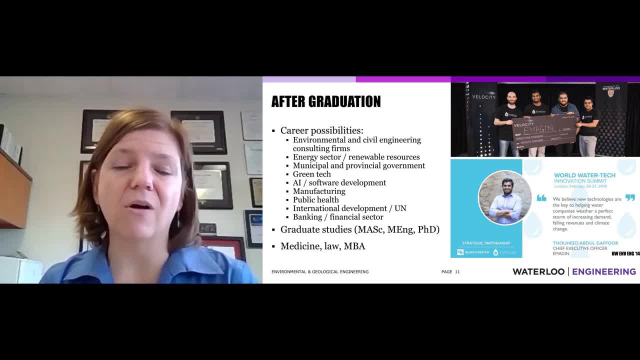 recently sold for an excess of 300 million dollars a few years back so these are global leaders and Waterloo startup and all within a very short period of graduating so we are putting out not 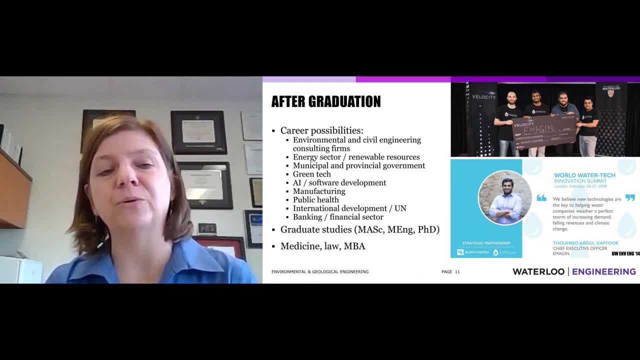 only competent technical experts not only competent people who can go on and work in other professions but people who are literally going and changing the world and in this case in climate change 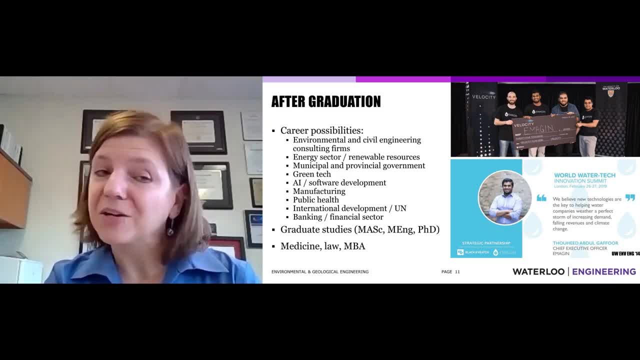 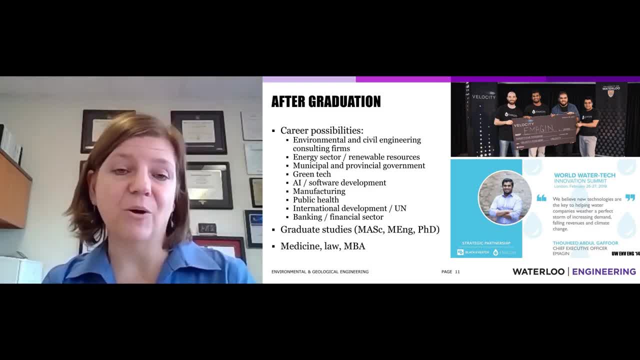 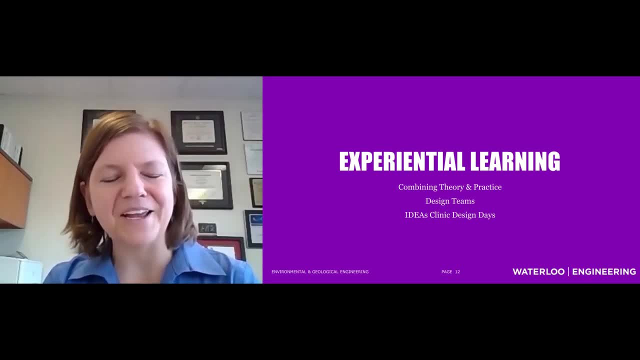 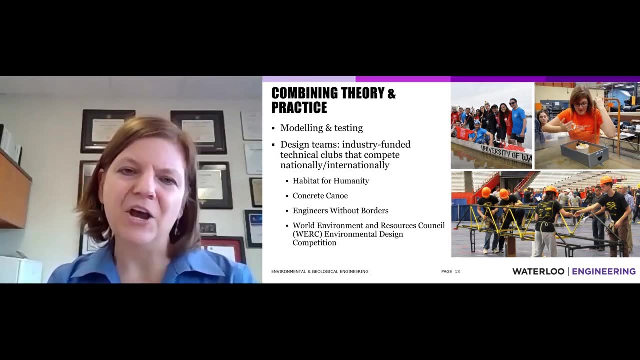 are the people who come back and interact with you within the program and that's where a lot of this experiential learning comes into literally practice and and also play so a big part of our program is about combining theory and practice the mind in the hand modeling and testing what 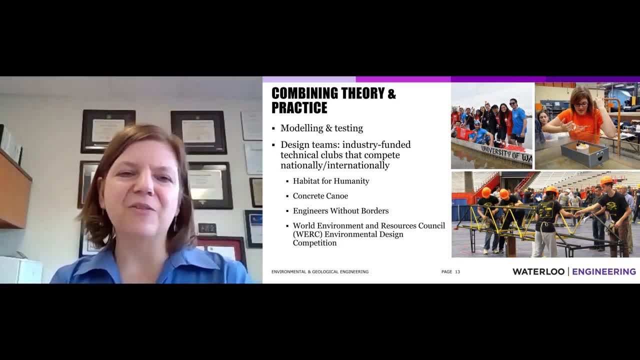 can we dream up and then how can we make it happen and that comes into play in the classroom but it comes into play in a lot of design teams if you can imagine it it probably exists here we've got habitat for humanity uh engineers without borders is actually where uh or actually originated here 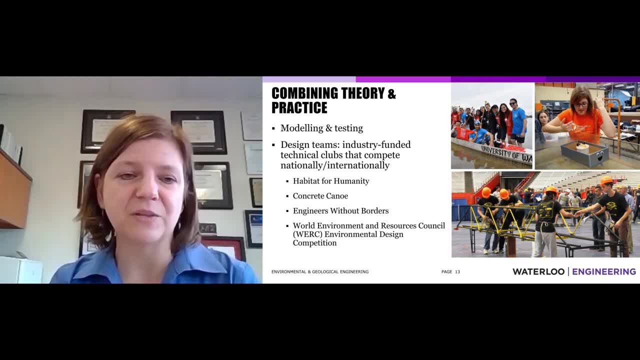 in Waterloo we've got many students involved in teams for engineers without borders and just because you're an environmental engineer or geological engineer doesn't mean that you can't get involved in other teams like concrete canoe a lot of our students get involved in concrete canoe 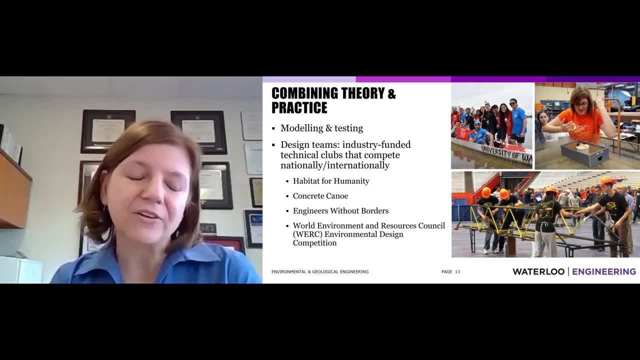 steel bridge design um also the water environment and resources council environment and environmental design competition so again you've got the skills it's a question of where do you want to apply them and where do you want to expand on your day-to-day activities in the classroom one 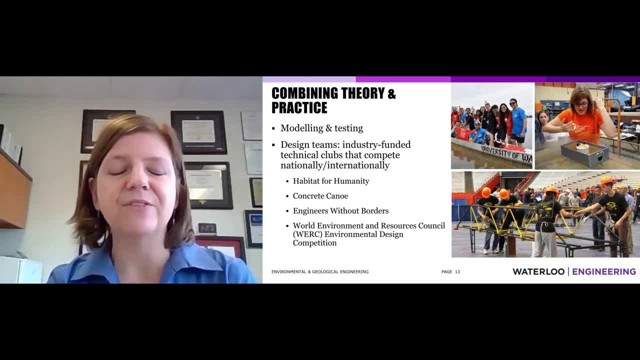 of the nice things that I can say as a course instructor is also when you have these opportunities to participate if these opportunities take you beyond campus if you're involved in competitions there's always opportunities to integrate that with your coursework so it doesn't interfere now we do these outside things but of course we do a lot of these kinds of things inside the classroom as well there's a couple of things that we do outside of the classroom that we do outside of the 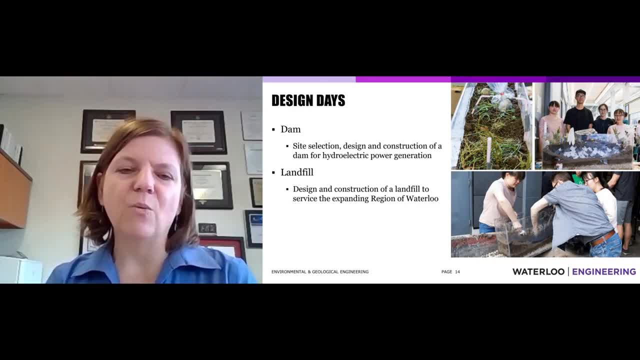 classroom as well so we have a couple of examples and images here from our design days program where we literally even early on in the program we like to think of our program as designed from day one across our department and you're starting to be exposed to those concepts really early on whether it be design design of dams landfills we always pick a topic that's relevant and industry experts come in and they provide you with feedback and ideas on how to grow that feedback into capacity 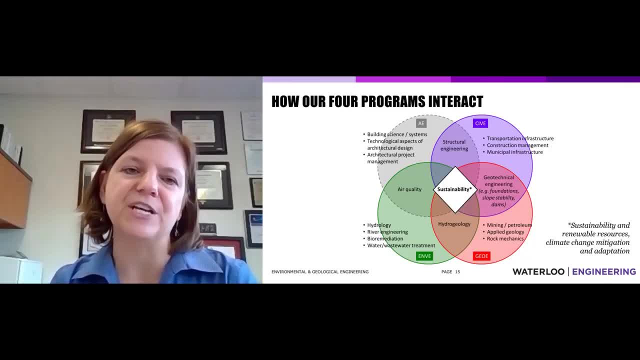 this figure just because i think it really nicely shows the interaction between our four programs 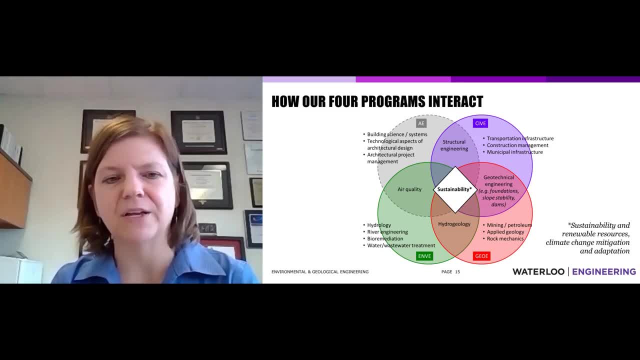 architectural engineering civil engineering and then the two programs we're talking about environmental engineering and geological engineering now i'm not going to read this 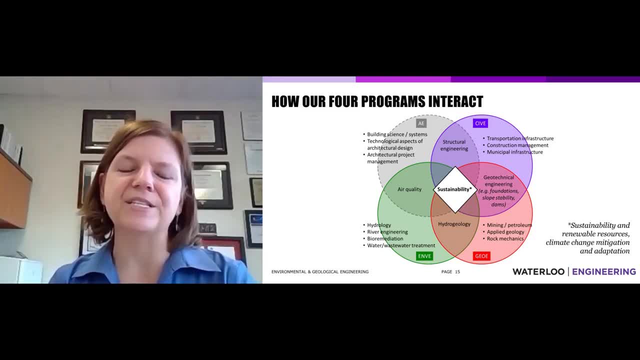 slide to you because you can read it yourself but the point here is that at the center of all of this is the notion of sustainability so sustainability is a boundary condition for all engineers so what we do is the boundary condition for how any engineering discipline is 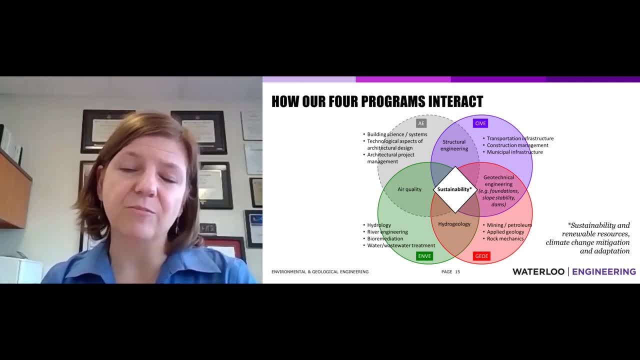 going to look at the interaction between people and the environment they live in it might be 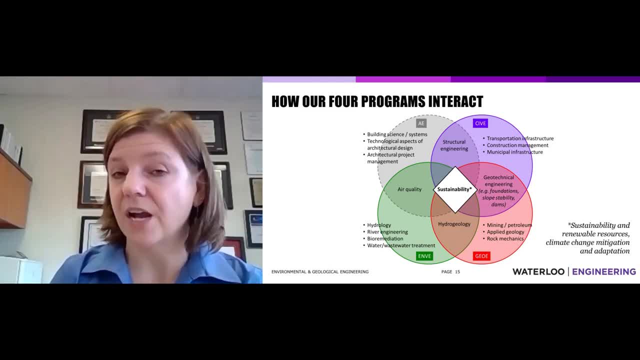 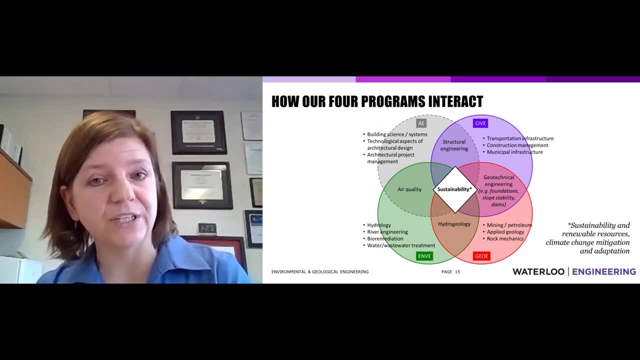 buildings and the built environment from that perspective which is more architectural engineering it might be the roads the bridges that define our communities and that's more civil engineering or 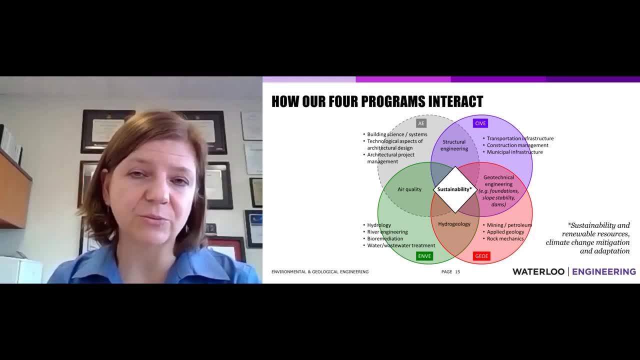 it might be the natural landscape our natural resources air land and water that's more environmental engineering and then geological engineering is more about what's 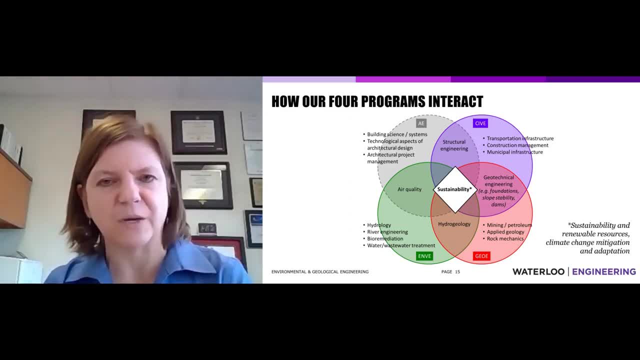 on our surface and our subsurface of our land and getting into that specialization but all of that boundary condition is necessary for humans to interact with the environment we 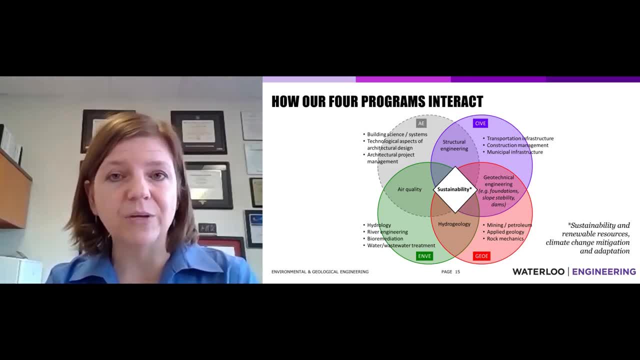 live in and now more than ever we're needed because that environment is affected by changing climate 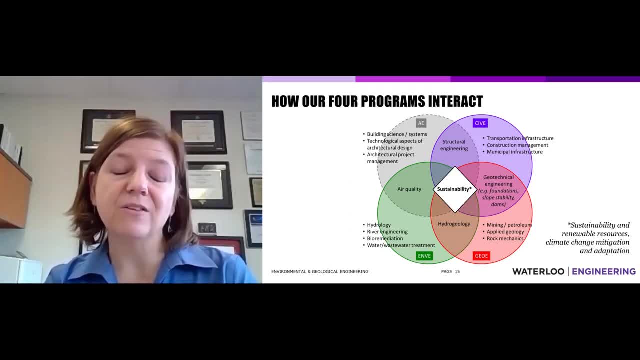 again floods fires we're interacting with the environment in a different way than we ever have before and so we have to have social хочет for all of these different issues and we have to have social supports for all five of them i think that's that's a powerfuleria office it's a yummy one and recover go ahead and have a ear if you want to hear more i know that there's just a couple minutes left this prequel so i think we're gonna go ahead and we can start here we're going to have the audience touch 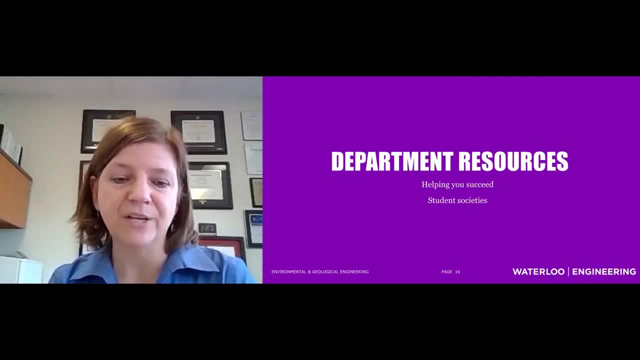 need to interact with it sustainably because it needs to be there not only for us now but also 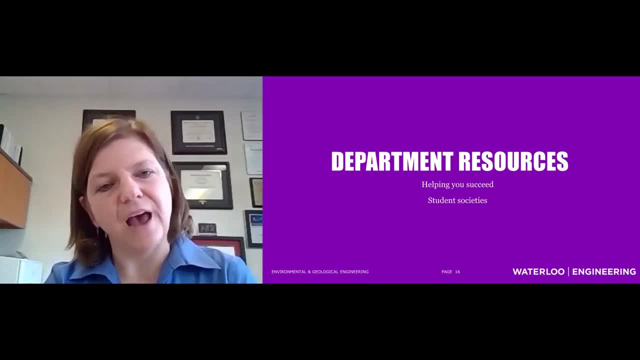 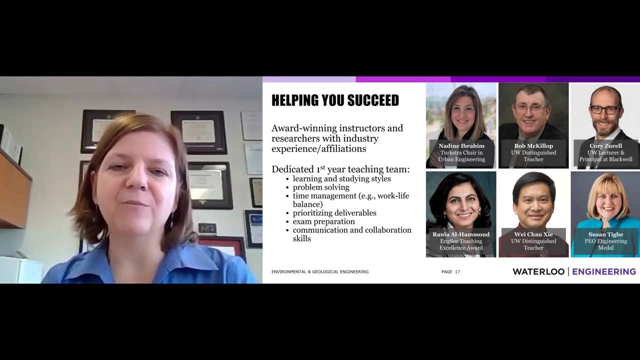 for generations to come in the future and so how do we make that happen with respect to departmental resources and the curriculum we've got industry leaders we've got academic experts and all of them bring that experience and expertise to bear inside of the classroom one of the really neat and special things about the university of waterloo's department of civil and environmental engineering is that we have a dedicated first year teaching team these are people who have won awards for teaching and they're not just here to teach you in the classroom they study learning and teaching styles problem solving they're here to help you manage your time to transition from high school to university we also have specialized tas who are students who are just a few years ahead of you that will also help you in the classroom with respect to managing your courses and your time because they've been there they can 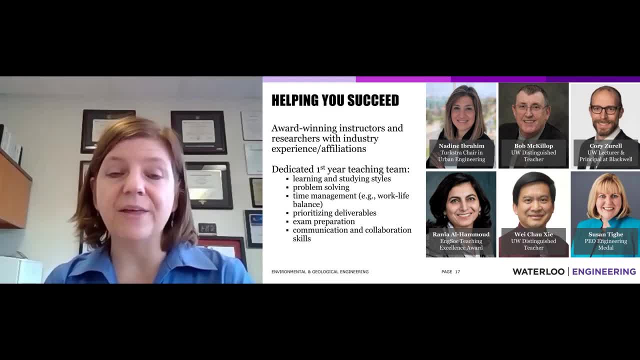 help you study they can help you prioritize your deliverables and they can also help you 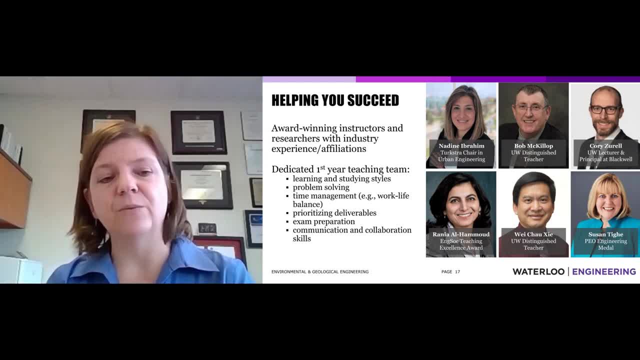 communicate not only with each other but with your instructors and with the administration to make sure that the program is advancing in a way that allows you to put your best foot forward because that's what we want we want everybody to do well and if that means changing things communicating and with how we interact that's what we're committed to doing it's a team effort here and 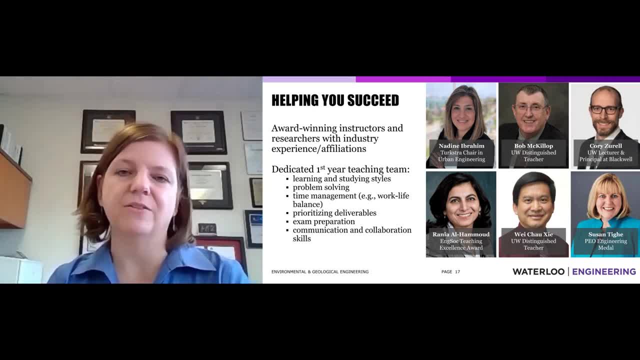 it's an open door team effort so anything that's going to help make the learning experience better all around 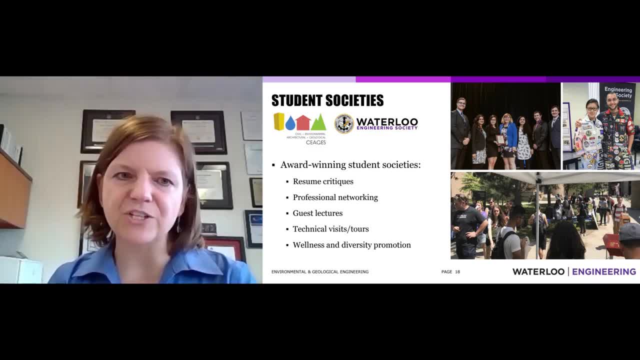 and part of that also then comes from how we interact with each other outside of the classroom we have a lot of award-winning student societies here we're 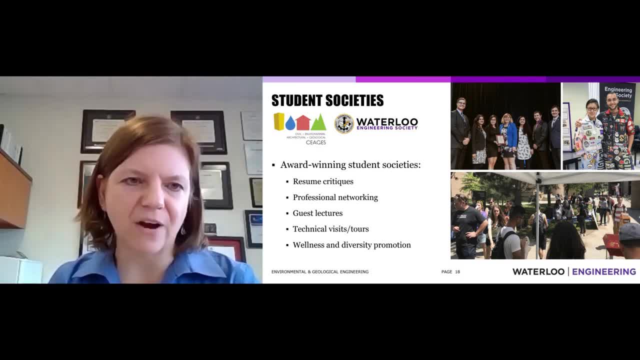 really proud of kegs which is the civil environmental architectural and geological engineering students group they're a perfect example of how we have these different programs in different disciplines but they all fall under the same umbrella and they're all charged with 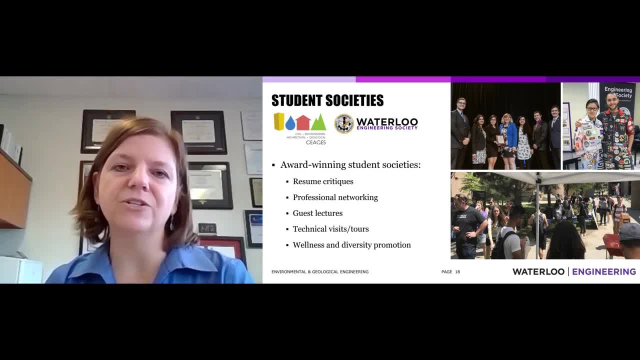 the same general mandate which is sustainable leadership in the environment of mindsets in this program how do i make sure that the language is indexed attached to the environment of mindsets trying to make sure that the language doesn't just get sort of 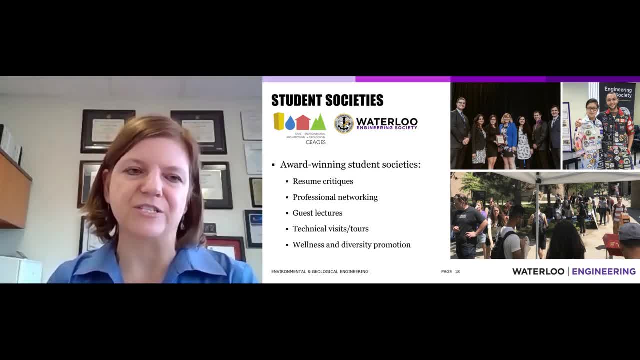 fully localized but goes through everything yeah it's great idea i love possibly to really 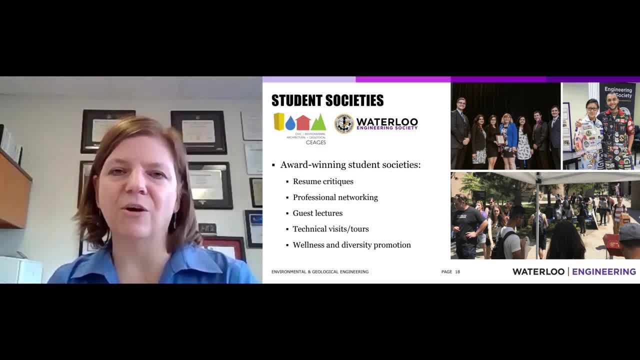 take a look at things one-on-one which we tried before and i hope will be a lot of fun it's working there now i'm going to give a brief introduction to the four groups i think you saw the first 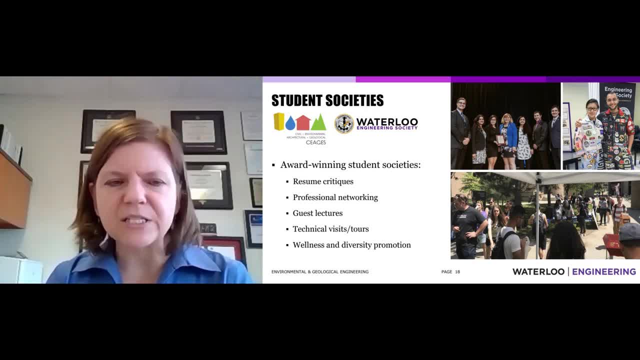 reason why it matters easy so for me one of the most common questions is is uh is you can do interviews and sixthss articles which is also something i've been doing for some time as a student so ilogize everything a service student does or i'm sure a lot of uh our student would use them a lot as well so i i'm sorry to cut this part because these things are pretty terminology that we're 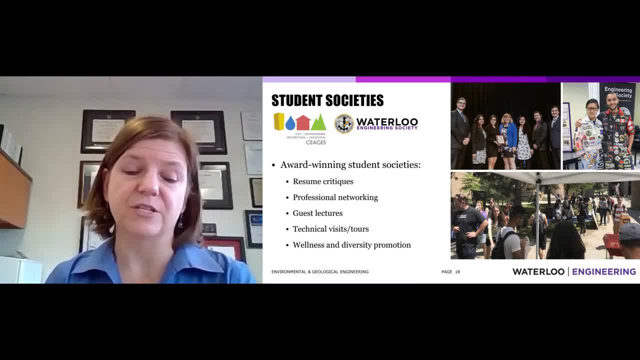 this topic, and it's not something we covered in class, we have guest lecturers that come in to talk about those topics. 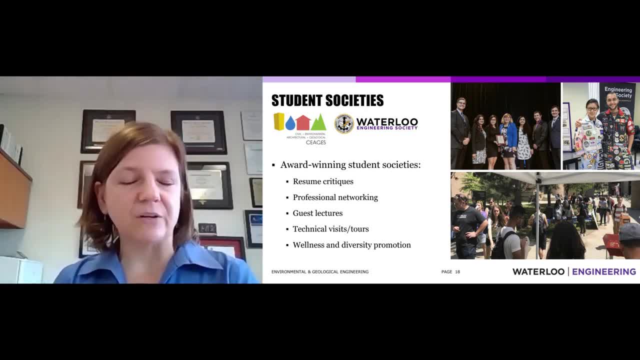 We have field trips, tours, et cetera. And of course, we're also very much committed to people's wellness, making sure that you know you're a person first, your health has to come first and foremost, and yes, there's the academic program, but it'll always be here. So let's make sure that you pursue it with putting your best foot forward and making sure that you're in the best place possible to continue down that academic path now, and then also when you leave here. 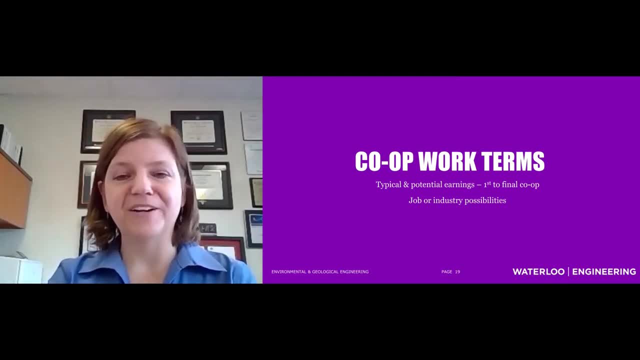 One of the things Waterloo is really well known for that probably isn't a surprise is co-op. So let's talk a little bit about co-op. We talked a little bit about co-op with respect to advancing through the program and how we pretty much alternate every other term, academic term in the classroom, then experiential term out in co-op. And the progression here of sequence is provided. 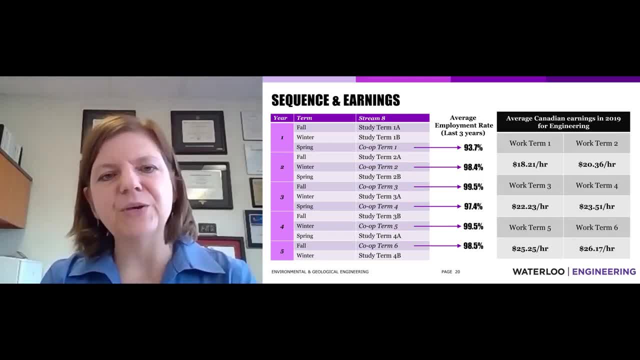 But one of the things I wanted to point out on this progression is you can see here, we have a really high co-op placement rate. It ranges here on this particular slide, anywhere from about 93.7% to pretty much full placement at 99.5%. 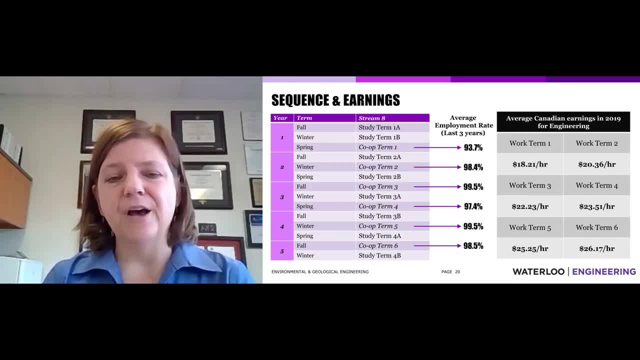 Employers seek out our co-op students because of their capacity. 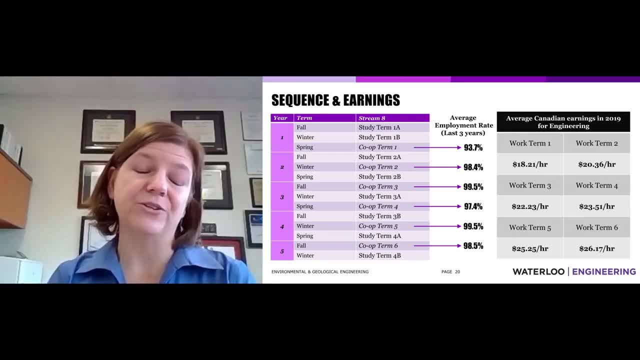 There's no question about that. The reason probably why our numbers aren't right at 100% 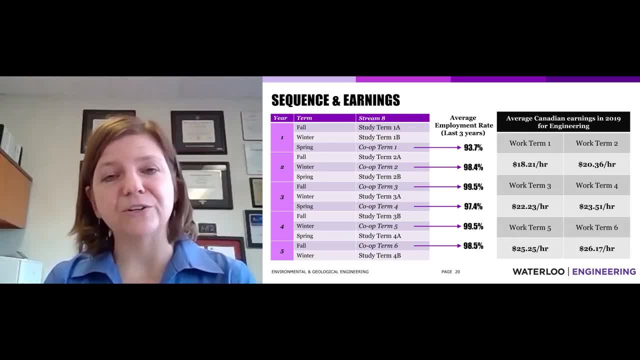 is because we have students that also go on their own terms with respect to opportunities, for example, for international study abroad, or they take leaves to pursue a competition, for example. And so they step away from a co-op term. We do have in our program a large number of required co-op terms. 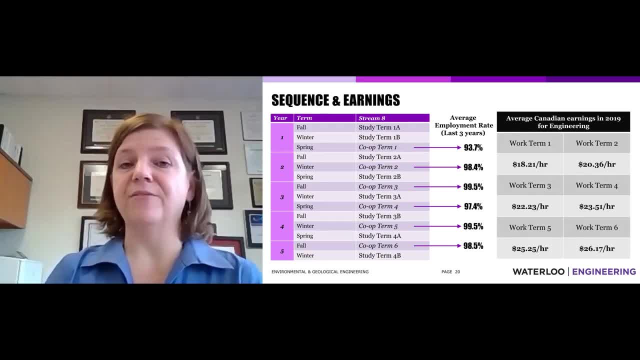 There are five required co-op terms. But you can have a sixth term where you may be on co-op or you may be doing something else. 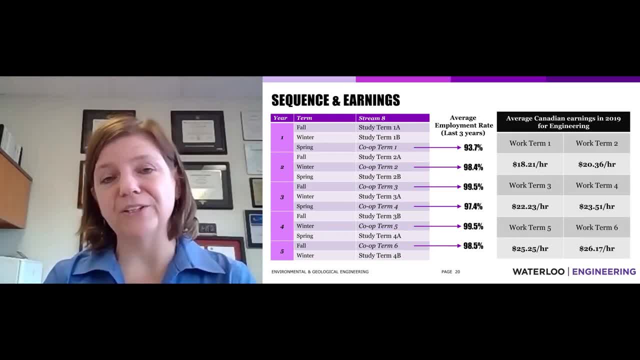 But regardless, as you can see from first year all the way through the final year, we have great placements. 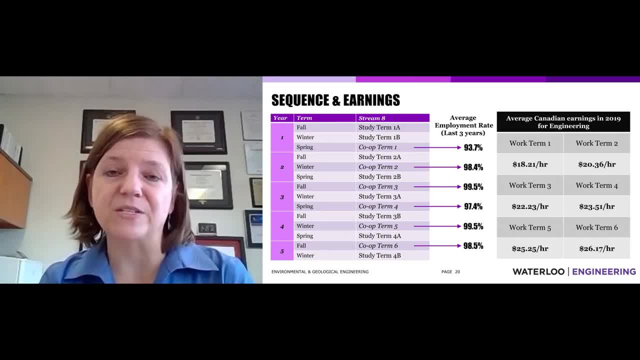 And we get paid very well as co-op students. You might have heard that students sometimes graduate from Waterloo with occasionally no debt, but probably more realistically, a little bit of debt. 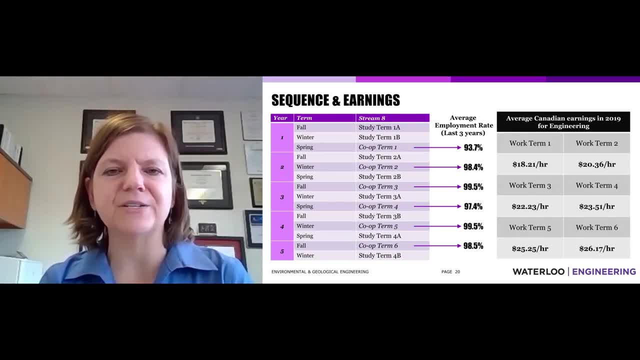 But as you can see by our average salaries or earnings for 2019 in engineering, our students tend to do well. So it allows us to think about how we want to manage those debts and perhaps 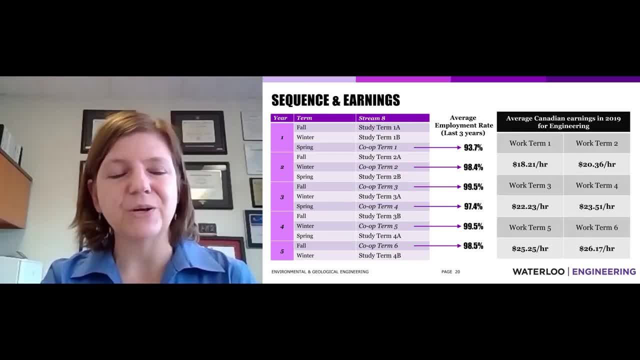 contribute to our education and the cost of that education. So students do pretty well with co-op. It's a great program. And to boot, you get experience. Thank you. Thank you. Thanks. Thanks, Rhonda. Hi. Hello, everyone. 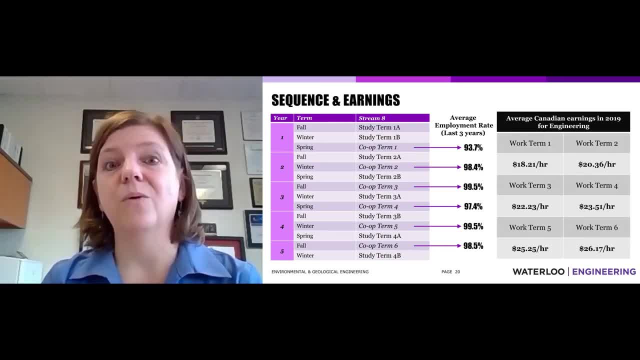 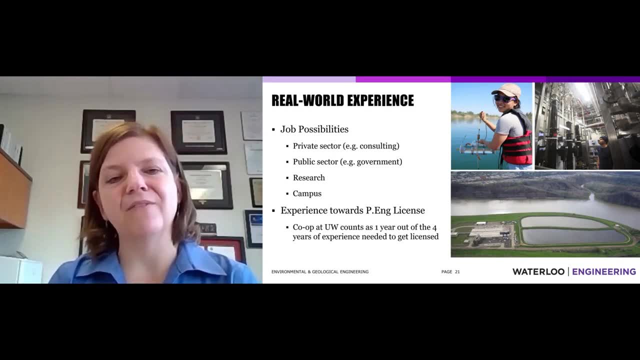 So I would like to briefly talk about some of the experiences that will help you decide not only what you do want to do, but equally importantly, what you don't want to do. So when it comes to those real-world opportunities, you name it. 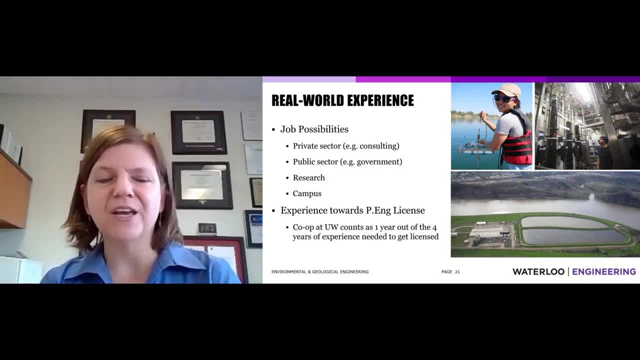 People have those types of opportunities. Private sector, consulting, industry, public sector, government decision making. 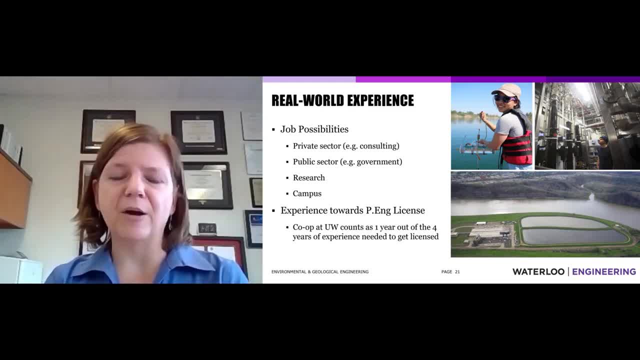 It could be regulatory government. But it also could be things like municipal government, 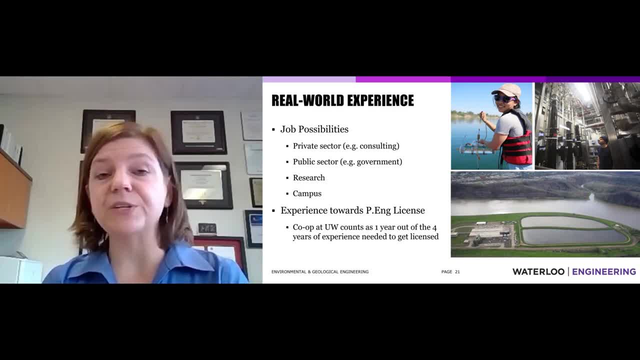 really depends on what you're interested in. Some people take research positions on campus, off campus. The positions might be focused on the technology aspects of environmental or geological engineering, or they might be focused on the landscape aspects, the natural infrastructure 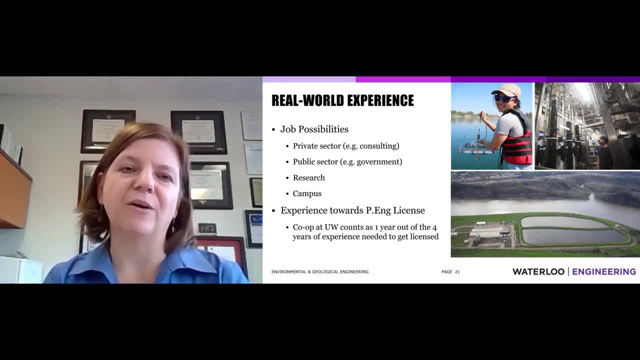 or environment that we're dealing with. One of the things I like to often talk about is I see it all as infrastructure. Some of it's natural resource-based, some of it is built, but it's all infrastructure that we're dealing with, and we're really negotiating how we interact with all of that infrastructure to maximize our goals and maximize benefit for society. But regardless of 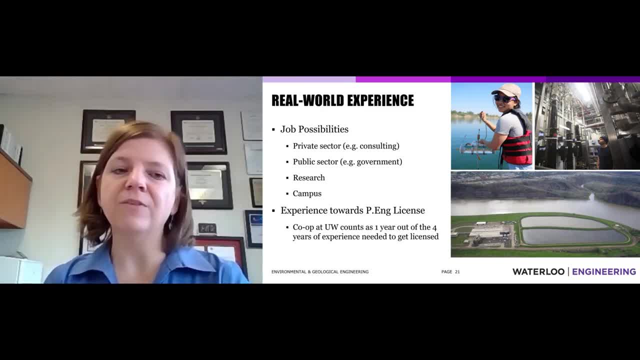 the types of interactions you have, the good news is that all of those experiences count towards professional designation. So P&G licenses, co-op counts as one year out of four for your professional engineering licensure. 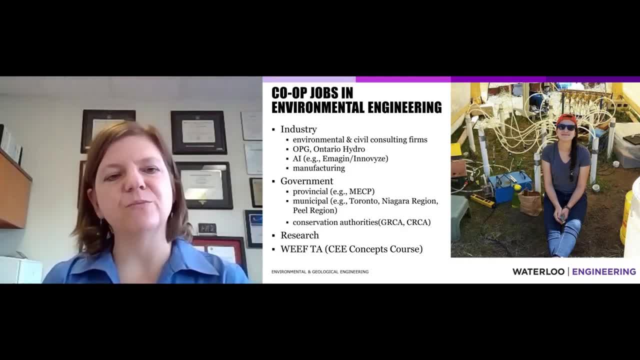 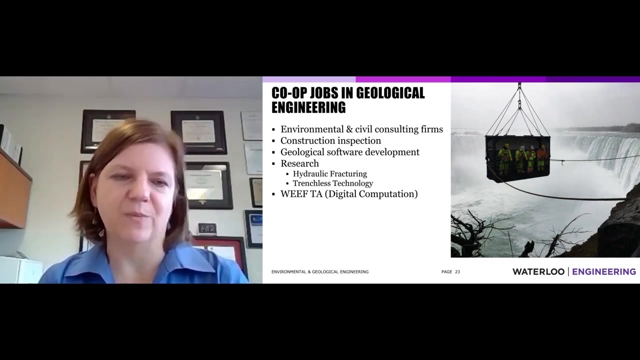 There's a whole range of jobs in co-op. I've got some of them listed here, and you can read them, again, ranging from industry, government, research. And one thing I'll point out is that you can also be on campus as a TA. So WEAP is the Waterloo Engineering Endowment Fund, and we have TAs. Those are those TAs I was referring to that help out first-year students. Those are our second, third, fourth-year students that are there to help share their experiences with you, and they're giving you a program because they want students to excel just like they benefited from other students who helped them excel. So there's a neat range of opportunities that you can have, and not only is that true in environmental engineering, it's also true in geological engineering. Some of them are more discipline-specific, but there's also those broader opportunities, environmental, civil consulting firms, the WEAF TAs, et cetera. So a really neat range of opportunities, and you can never capture all of that on a slide. 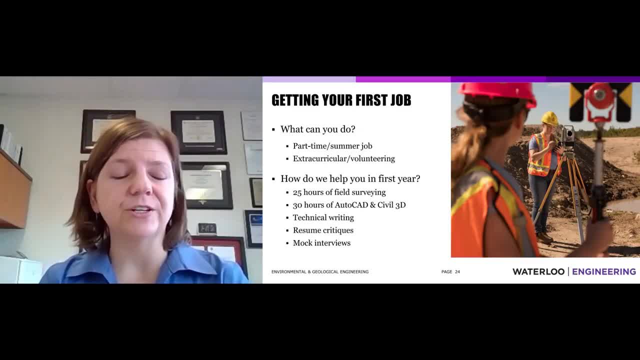 One of the big challenges is that you have to be able to do all of those things. So you have to be competitive, you have to be able to do all of the things that we now have the opportunity to do in front of you. But that's another of the big challenges that people ask us about is, first-year, 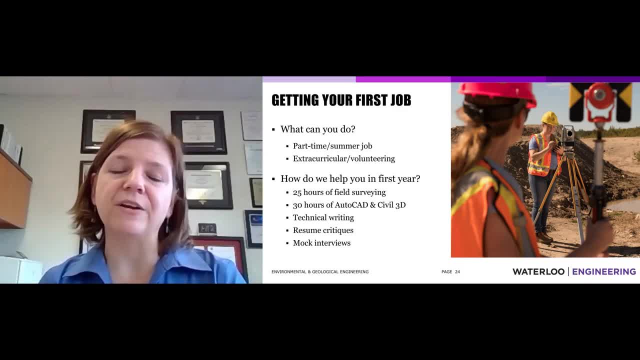 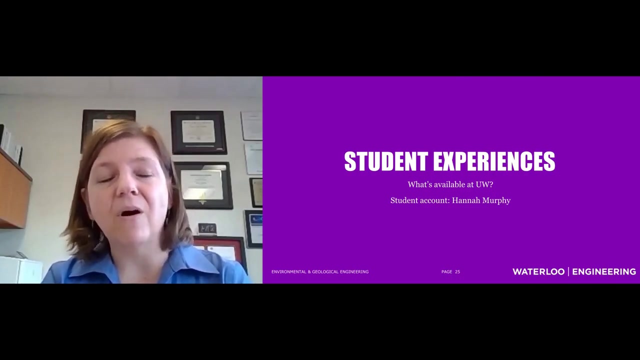 what can you do? Part-time summer jobs, extracurriculars, we really help you to get there with, in addition to having those experiences, giving you very specific experiences like surveying, AutoCAD, technical writing, in first year, in the first term, so that when you go out for that job, you're competitive. And not only do we do that from a classroom side of things, but we also do it from a professional development side of things as well, so we can have a really good side of things. So technical writing experience falls in there, but also resume critiques and mock interviews. Those come from both your professors and also a lot of the clubs, the student-run clubs we have on campus. And so hopefully, I'd like to think, but I think our 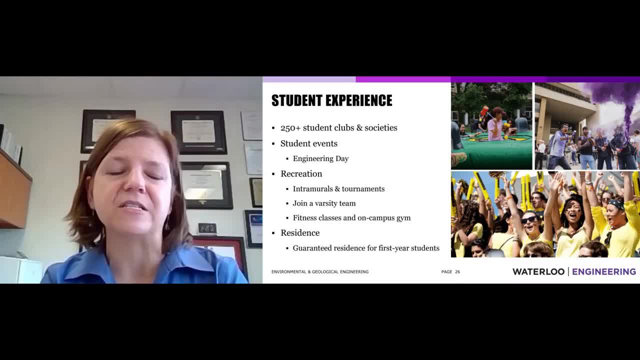 students think overall this leads to some pretty positive student experiences. So with over 250 clubs and societies, a lot of faculty, so engineering, faculty of engineering focused events, and then university-wide events, whether they be intramurals, varsity teams, just clubs, fitness clubs, and also residences that have their own activities. There is a whole lot to do here. 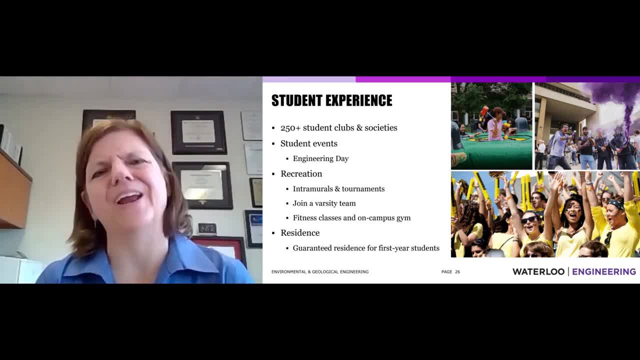 And I think if you talk to any UW engineering student, and that really goes for any discipline in engineering, but certainly in the programs we're talking about here, there's time for that. 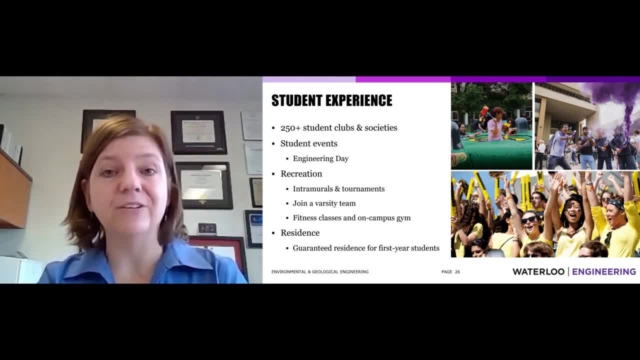 We want you to have time. If there's not time for you to have a life outside of school, that means we're doing something wrong. 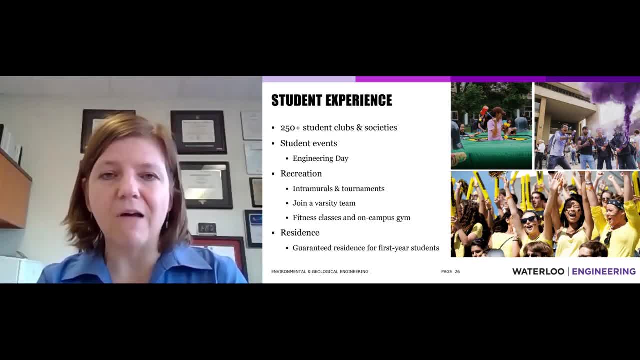 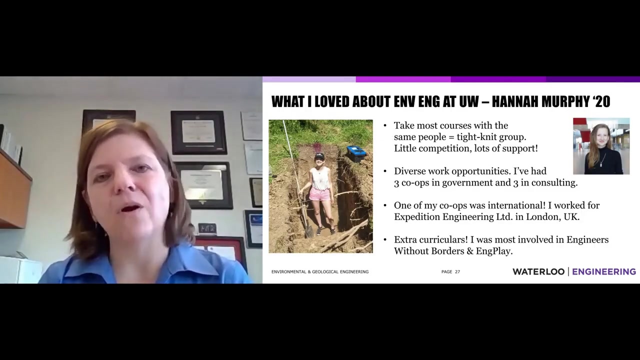 Because we're interested in people developing as whole individuals, not just as the narrow technical civil engineer, environmental engineer, architectural engineer, geological engineer. We're a group. It's family-style education, open-door policy, and we're committed to everybody progressing in areas that interest them. And you'll see this in what our students 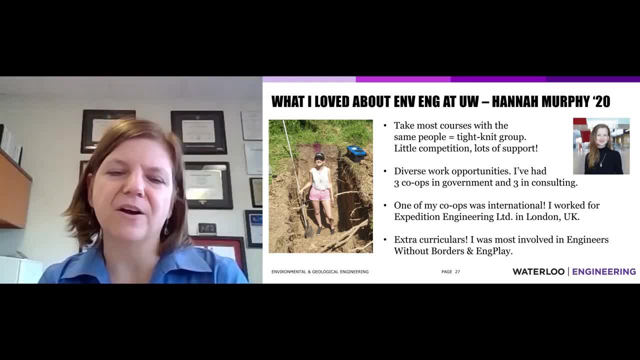 say. This is an excerpt from something that one of our environmental engineers put together by the University of UW. 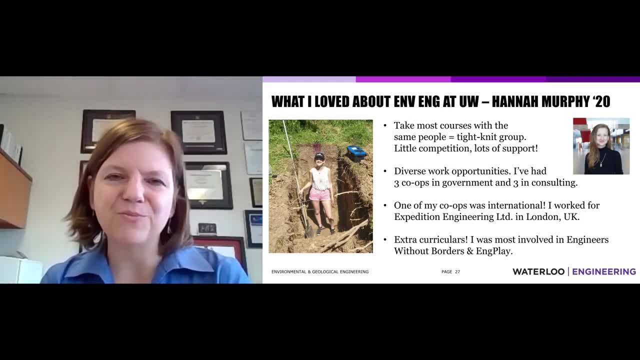 And it's about why I love being at UW. And her name is Hannah Murphy. She's from the class of 2020. And she talks about exactly these ideas, that we're a family-style tight-knit group. You take most of your courses with the same people. Yes, you can take different electives, but for your core technical courses, you're pretty much together with the same group. And what that means is little competition, lots of support. One of the things I say to my classes that I teach is I would be thrilled if everybody had above a 90. I'm a senior student. And we want you all to learn and we want you all to succeed. And we're committed to doing what it's going to take to help get you to that point. And that's inside the classroom and outside of the classroom. So there's diverse work opportunities. Hannah said she had three co-ops in government, three in consulting and one of her consulting positions was actually with a group called Expedition Engineering in London, England. So getting a very broad perspective and she applied that also into her day-to-day life. 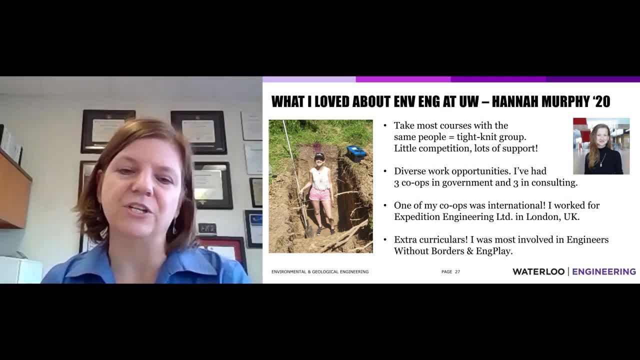 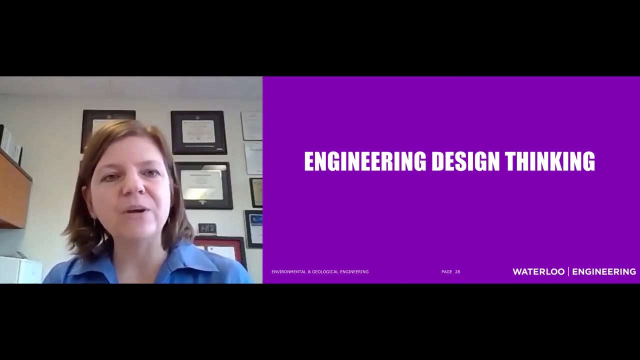 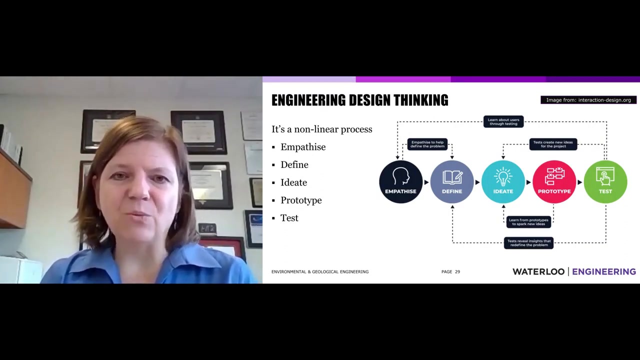 outside of the classroom, she got involved in a lot of extracurricular activities, which included EngPlay and Engineers Without Borders. And so there's really something for everybody. And we want you to come in and be part of this nice, small, tight-knit community. 80 people, and that's at largest, that's not a lot. The people here who are here, we want people who are good and technically, academically, but also who want to have fun, who want to get involved and be leaders and experience life, experience their interests. So go for it. That's who we're looking for. And that kind of philosophy really transcends into how engineers do things, how we do things. There's this idea of engineering design thinking. It starts with empathizing with people. So really understanding what the need of society is so that you can define the problems that need to be solved and then generate ideas to solve those ideas. 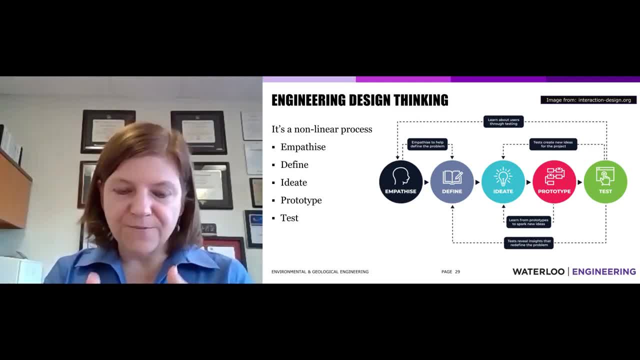 But then, be able to focus in and create a focused approach because we can brainstorm until the cows come home. 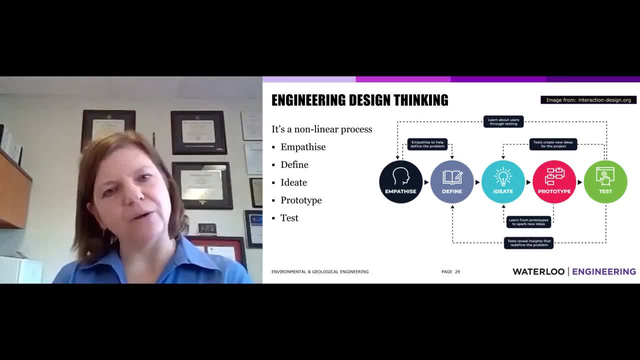 But how are we going to get to those actual solutions? Then we go out and test them. And then we sometimes have to iterate. We have to go through these steps again. And so the idea is 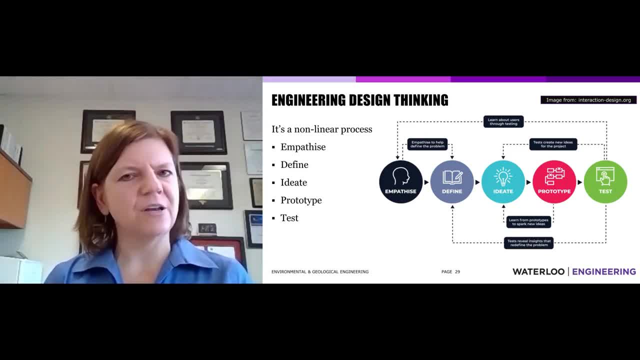 that this isn't a linear process. If you're interested in problem solving, it means you're interested in engineering often, especially if you want to problem solve with science. 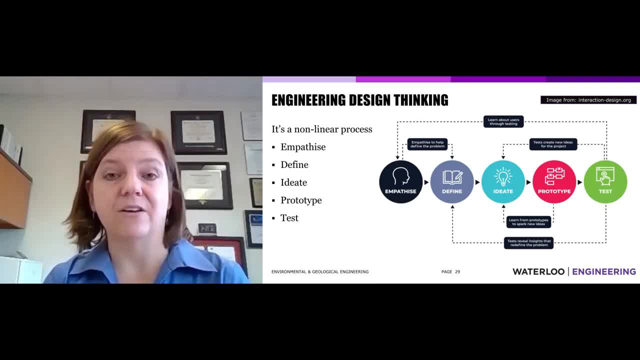 The question is, how do we make sure we actually have an end product that's going to have an impact for society? 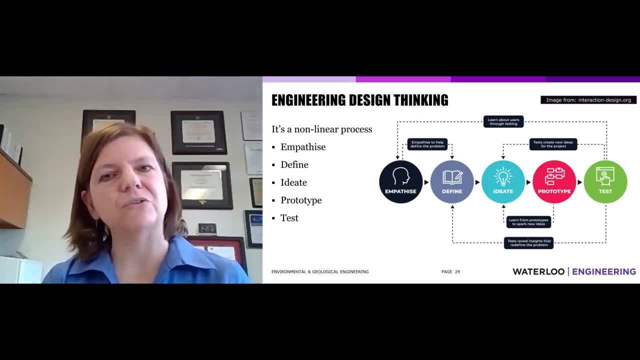 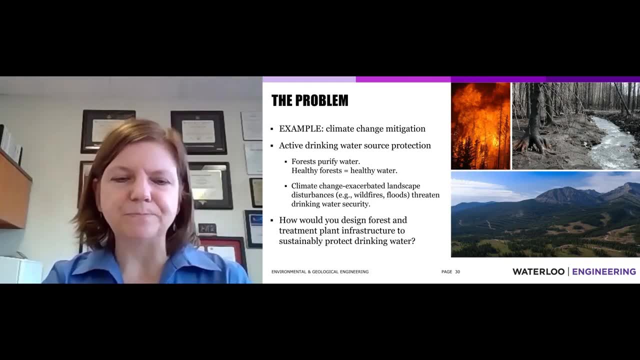 That's the engineering design thinking process. And that's why engineers can do so many things career-wise outside of the engineering discipline, because it's about problem solving. And so I have a little example here of a problem that I've been really involved in. It's climate change mitigation. 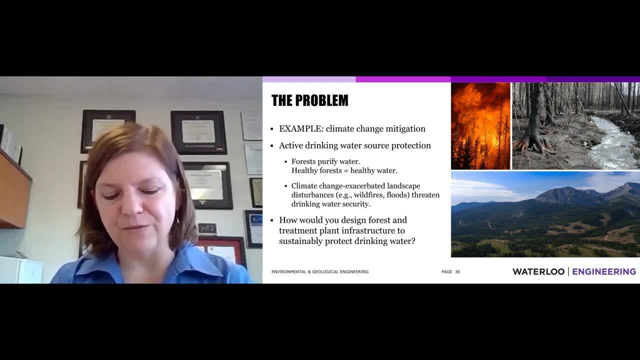 And I'd really describe it as climate change mitigation and adaptation. We've got students ranging from high school through PhD students, so doctoral students involved in projects like this. 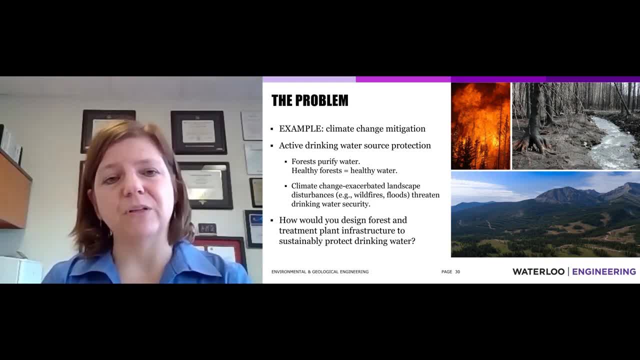 So the question is, how do we protect our drinking water supplies from water pollution? From climate change exacerbated landscape disturbances. You think about what's happening recently in Australia. Wildfires, floods. If you look at what they do to the landscape, they punch well above their weight class with respect to potential detrimental impacts for our water supplies. And so the question is, you know, we can't prevent those. We can try to mitigate those disturbances, but we can't prevent them because climate change is here and it's happening. 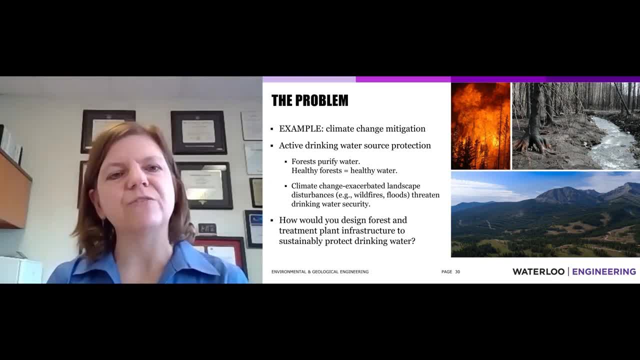 So how do we mitigate and how do we adapt and what can we do moving forward? And so part of our work has focused on, well, the majority of our water across this country, across many parts, the world comes from forests. And if we can have healthy forests, we can have healthy water supplies. And so the question is, how can we look at that forested environment and what can we do actively? Not these passive policies of don't contaminate, but what can we actively do to nurture the landscape to nurture that natural infrastructure, to make it work as well as possible so that we have healthy water supplies um so it comes from moving back and forth and saying well if you're in a place like alberta well in alberta that's a wildfire prone landscape if you're in a place like halifax nova scotia well that's hurricane prone so the risks to the forest there are going to be blow down as opposed to burning of the landscape and you say okay well if we know that then how might that affect water and how might that affect our ability not only to have a clean water supply but then what infrastructure do we have in the built environment how is that change in our water supply going to affect how well our built environment works and so you can see this iterative process where we're going back and forth and really understanding what's happening on the landscape and what's happening in the built 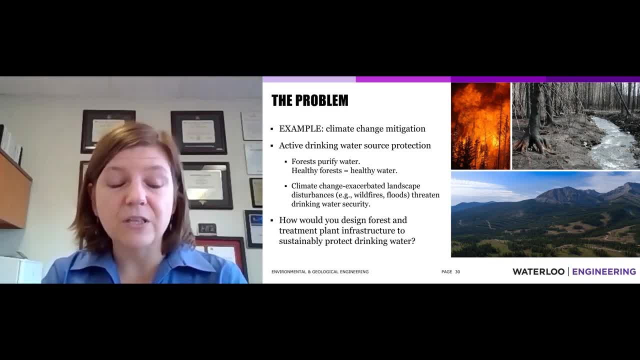 environment to achieve targets of society which in this case our public health protection because if you don't have safe drinking water that's when diseases really start 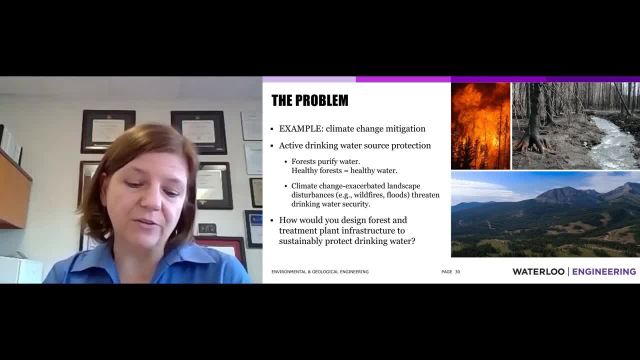 to grow in society and this is something you might have heard about with hurricane maria or other disturbances that have happened on the landscape recently this is probably something you most 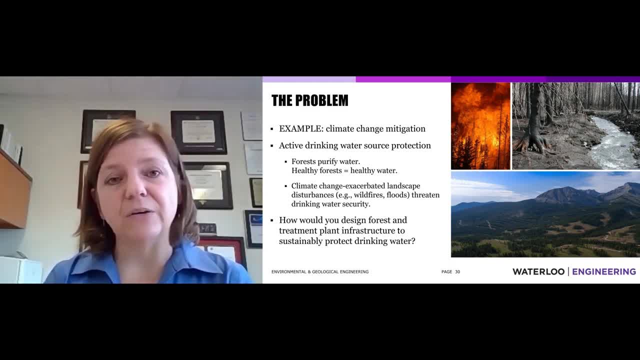 recently heard about in australia and you might not be surprised now to hear that we've got groups from waterloo providing guidance not just across this country but also in other areas like australia